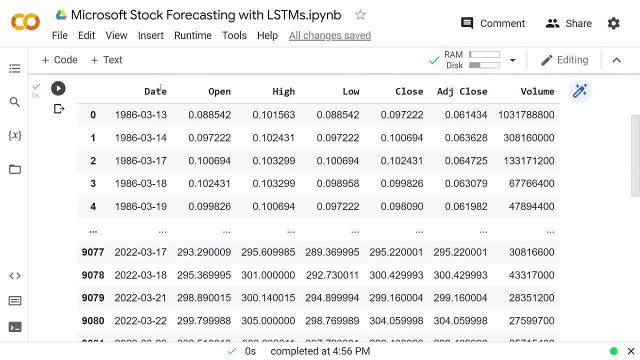 Looking at the different columns of the dataset, we have the date and on that date, what the stock opened at the highest value for that day, the lowest value for that day, what it closed at the adjusted closing value and then the volume of stocks traded that day. We're going to keep. 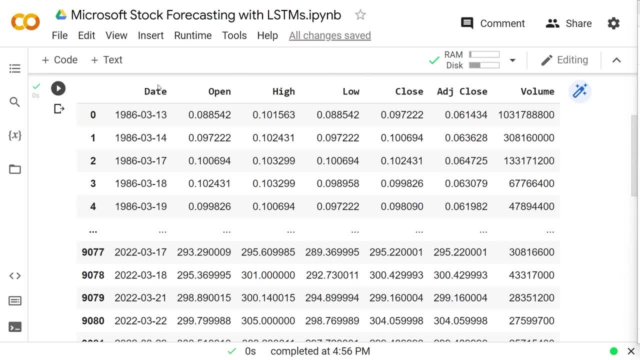 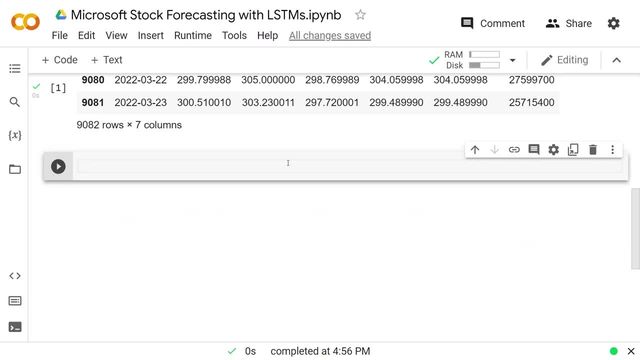 things simple by just using the closing value. so we'll have the date and what that value was at the end of that date. We're going to keep things simple by just using the closing value. we're going to discard the other columns. We can do that by doing: df is equal to df and just the. 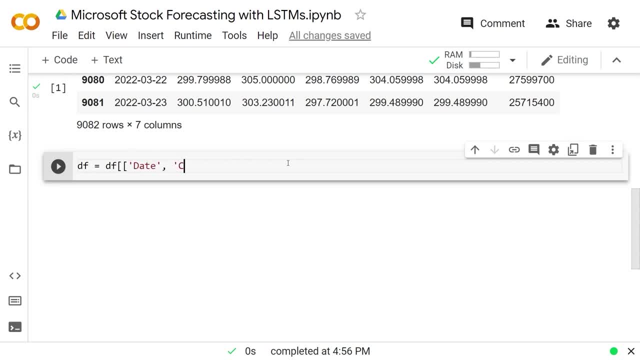 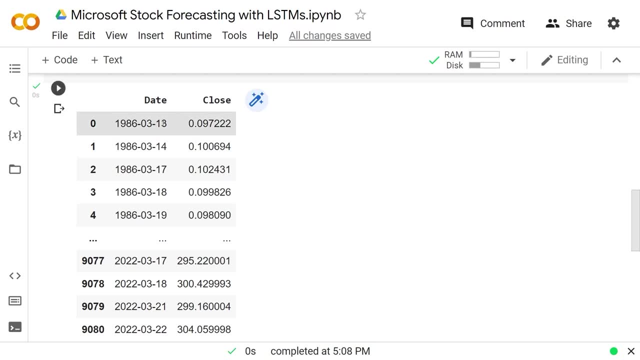 name of those two columns, which is date and then close. We'll set that and then, outputting df, we should see only those two different columns. We currently have a problem with our date column, as it's actually not a date, It's just a string that has the year, then the month, then the day. 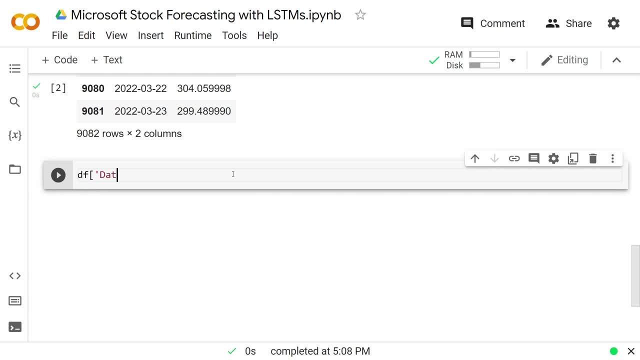 We can see this. if we type df sub date, we should see name of date. except it's a d type of object. We want that to be a date. We usually use this thing called date time, so we will import date time and then make a function. We will define a function called. 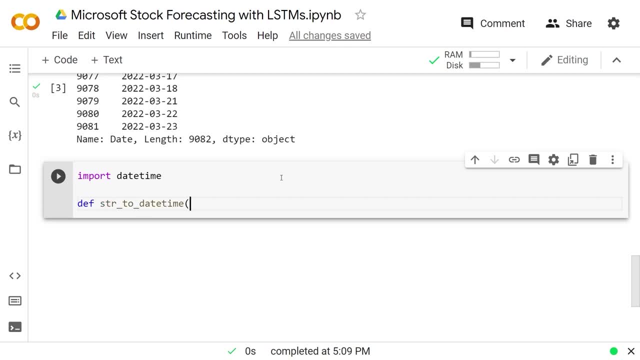 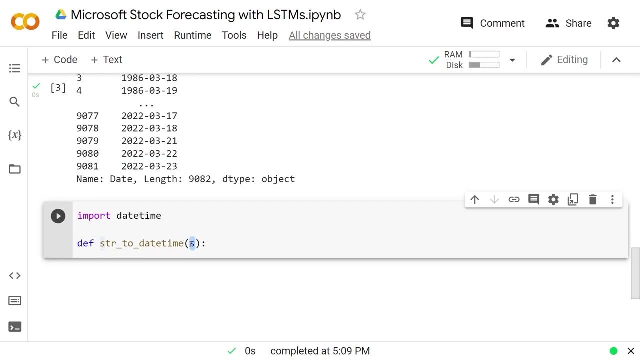 string to date time which is going to take a string s, which will be any of these strings here, any string that looks like this: We're going to pass that to the function in s and it's going to return the associated date time for that string When this function will create a variable. 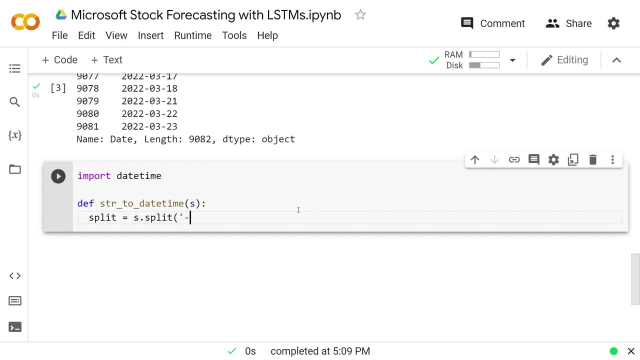 here we're going to set that equal to the s dot split. the hyphen, which is the separator for each of these A split, is going to be the list of the year and then the month and then the day We can. 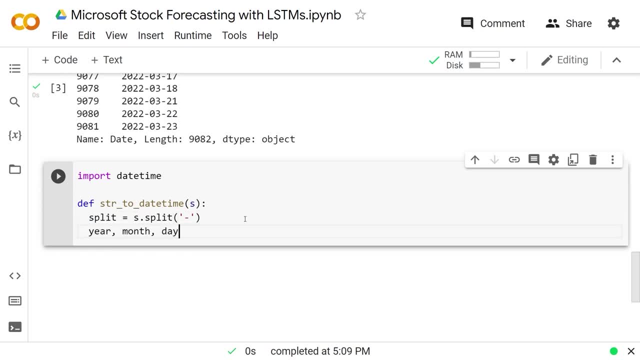 extract those three pieces: year, month and day, equal to the split of zero, split of one and split of two. These objects are actually strings. right now We want to make them integers, so we'll just wrap each of them in int. 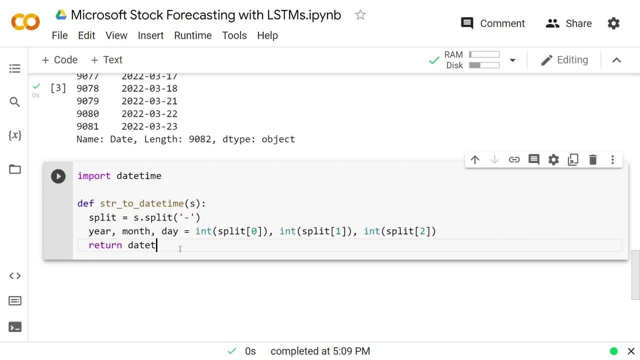 So we can just return the date time, dot date time and then pass the year equal to our year, the month equal to our month and the day equal to our day. We'll now test out our function by creating an object called date time underscore. object equal to the string to date time. so 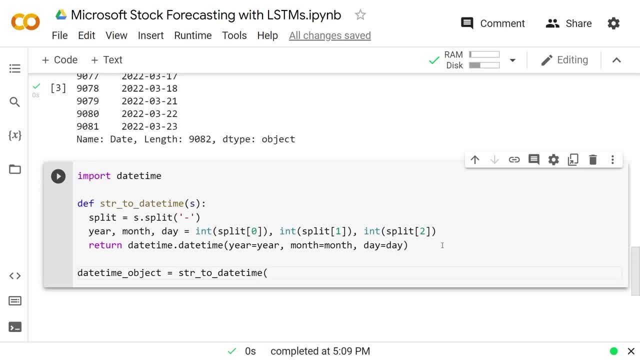 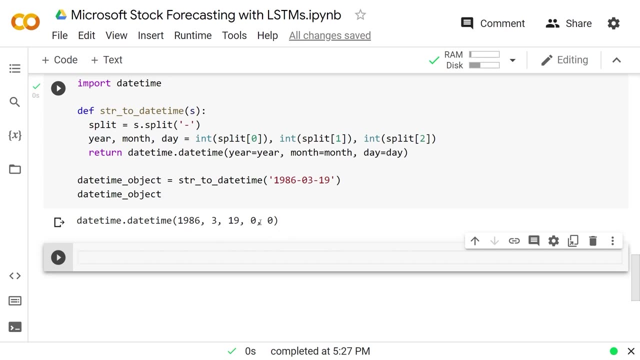 calling our function and we'll pass the first day in our data set, which happens to be 1986-03-20.. If we output this date time object, we should see that it outputs date time dot date time of 1986-03-19,. and this is for the time. but we don't need any of that Now. what we need to do is apply. 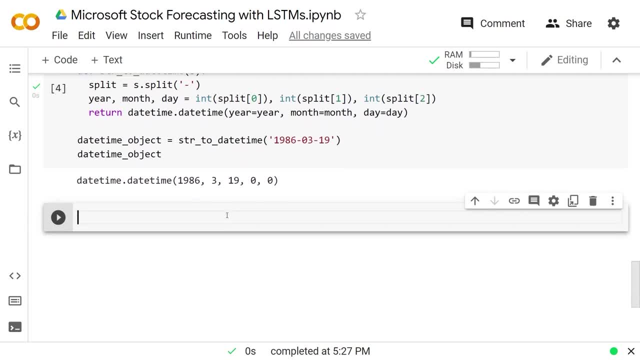 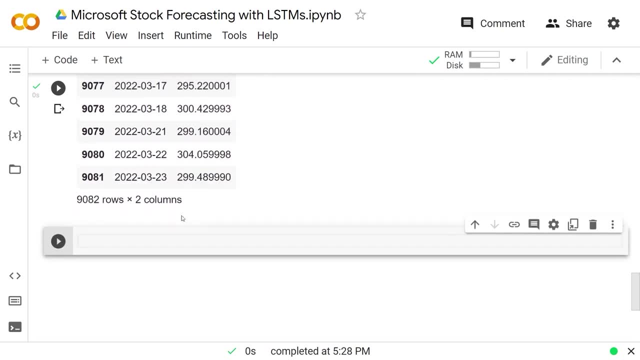 this function to everything in our date column, because we have in df this whole date column. we want to make all of these date strings actual date objects, So we'll set df sub date equal to itself. so df sub date dot apply. We're applying a function to that column, just the one that we made above. We can pass string to. 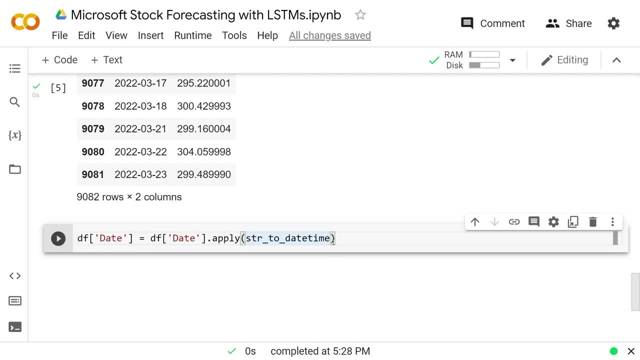 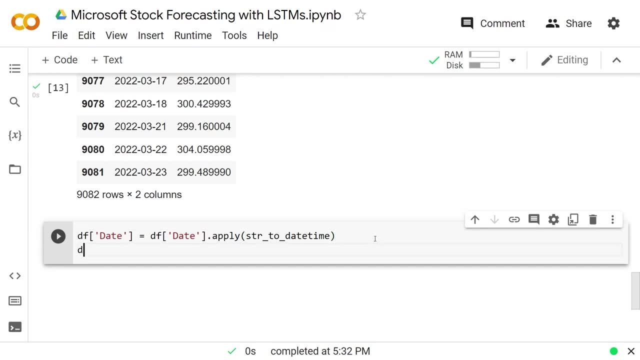 date time into this function. Note that we're not calling the function here. we're passing the function itself to the supply function. Now, if we were to output our data frame column again, df sub date should now show us the following: It looks like this is an error, but this is just a. 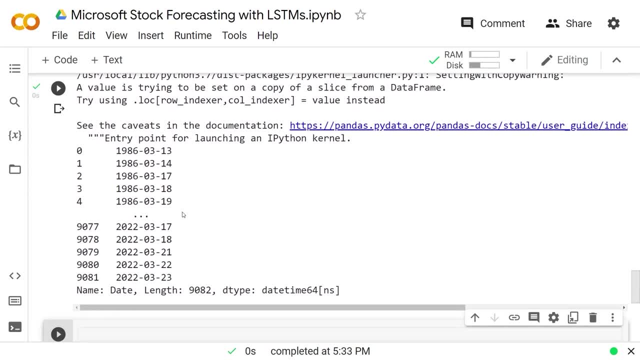 warning. this is okay. It looks like our column is the same as it was before, but actually the d type is now date time 64.. This is the same as it was before, but actually the d type is now date time 64.. 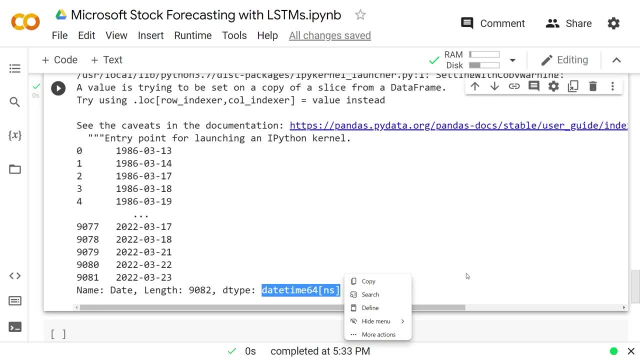 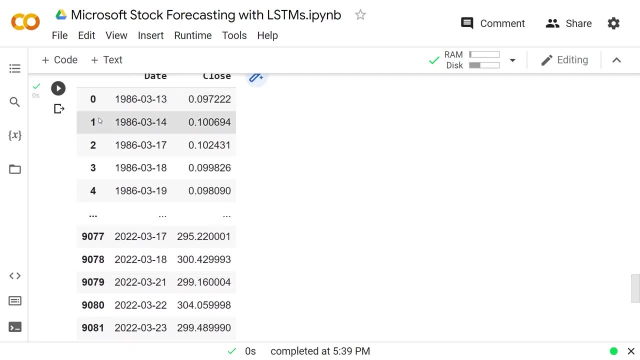 This is just what pandas converts it to. this is actually what we want. Our data frame is almost ready. we just have one more step. If you look at df, you can see that it's index. this column right here is actually integers. We want to replace that column and make 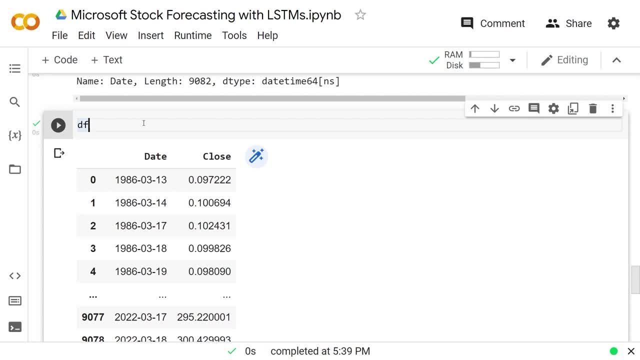 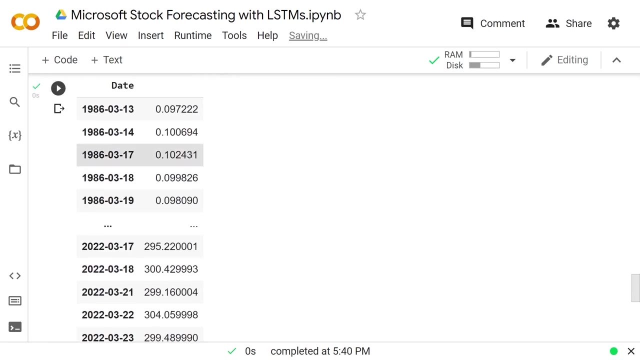 that date column the index. We can do that very easily by setting df dot index equal to the df dot pop, which means we take away the column and return it. So df dot pop, passing the date and then outputting df, we'll see that it did exactly what we desired: Make that date column. 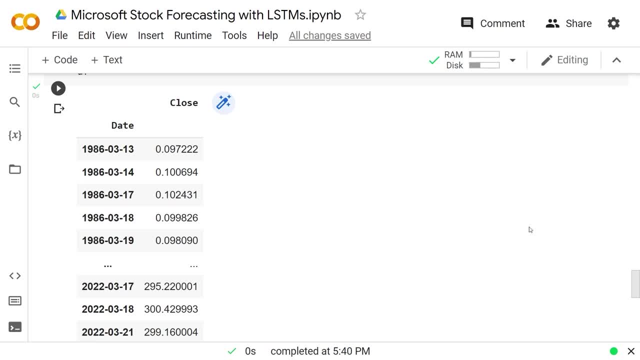 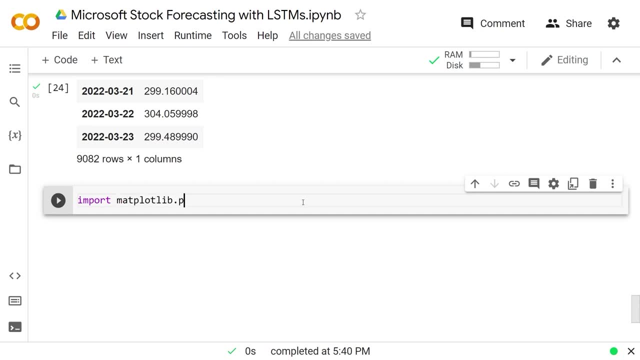 the index and then we just have the closing value as a column. Now that we did that, we can quickly plot our data using matplotlib. If we do import matplotlib dot pyplot as plt, we can do a plt dot plot of the df dot index and the df sub close. What we can see is from 1986 all the way up until 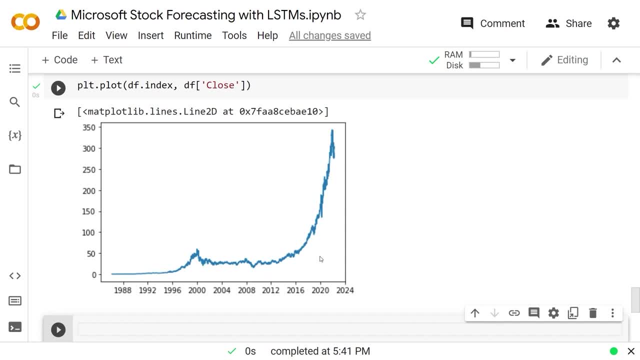 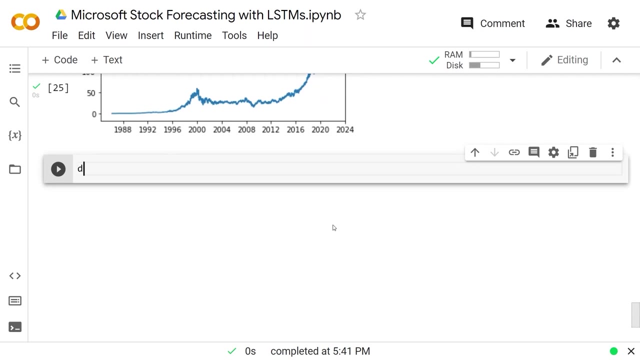 2022,. the stock goes absolutely crazy after it hits about 2016 or so, and then there's a little bit of a drop at the end. Now, because we're using the LSTM model, we need to convert this into a supervised learning problem. We're going to do this by making a new function. we'll call it define. 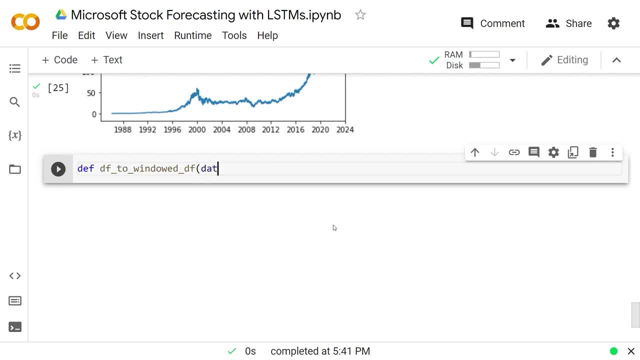 df to windowed df. It's going to take the data frame which we'll just pass df. it'll take a first date string and a last date string and then a positive integer. we'll set it equal to 3 by default. This function is also going to. 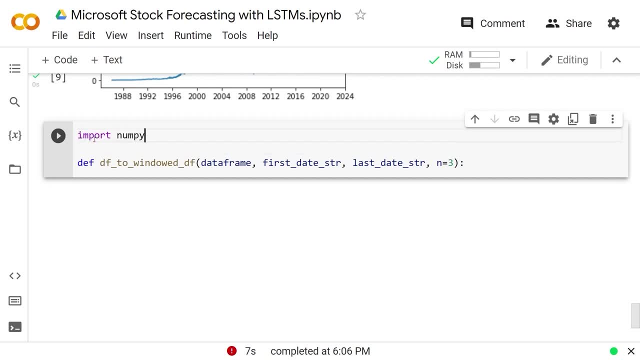 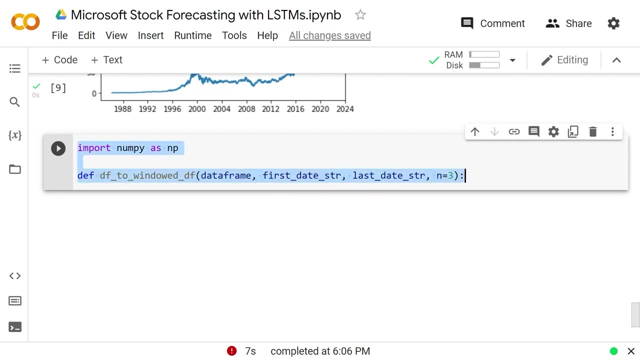 need numpy, so we're going to import numpy as np. Now it turns out that this code is extremely difficult to write, so I'm going to just go in here and paste in the code. If you need to know what that code is, make sure you go to the video description and check out the tutorial and look. 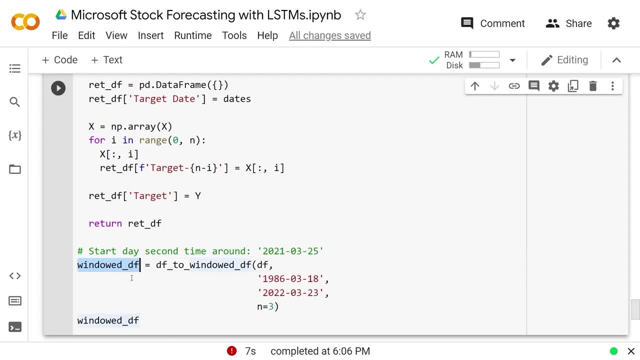 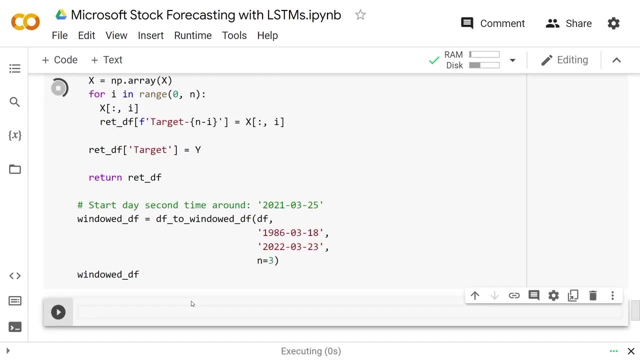 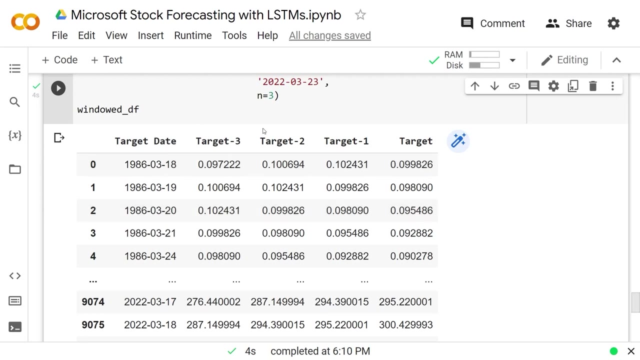 at it there. I also pasted in how to create this object called windowed df, which is calling this object. I'm going to explain that very shortly. I just need to show you the result of windowed df. Windowed df is now a data frame where we have a target date column, a target minus 3,, minus 2,. 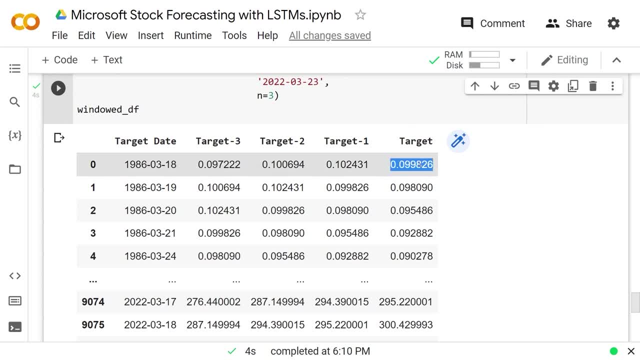 minus 1, and then the target. These are all the stock closing values from before, so this target date corresponds to that value here. If we look above at 0318, it should be 0.099,, so 0318, let's. 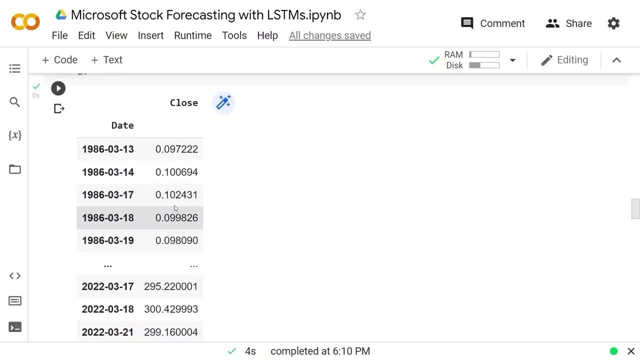 take it one more time for me to remember: 0318 is basically 0.099, so 0.099 is 0.099,, so 0.099 is 0.099, so 0.099 is 0.099.. Why don't we have this row, that row and that row? Well, that is all about. 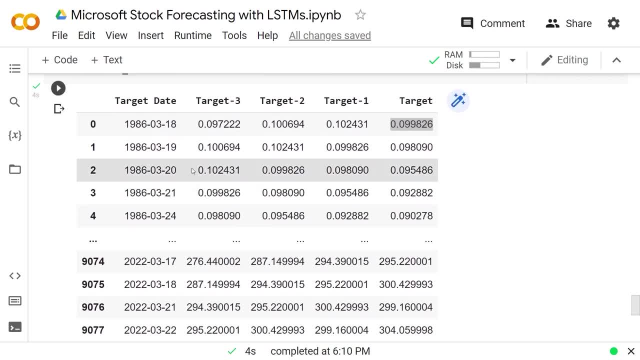 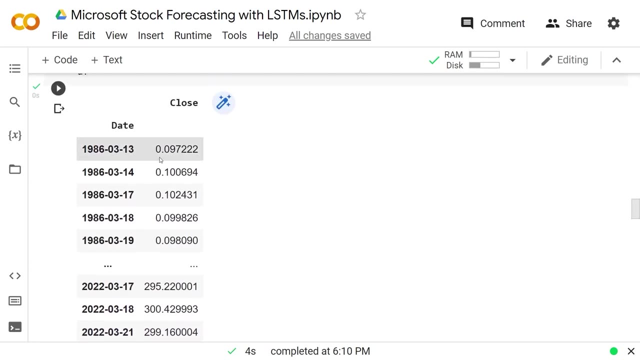 what this windowed function is. So this windowed data frame is converting a date into getting its three previous values and then what it actually was. So if we go back again 0.097, if we look at what 0.097 is, that is three days before This is the target date. this is three days before. 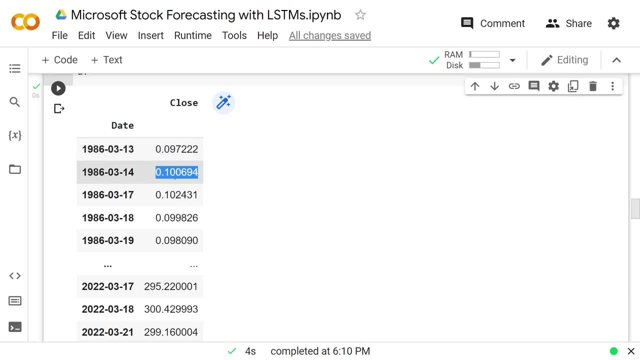 If we look at 0.097,, this is the target date. this is three days before. If we look at 0.097, here to look at target minus two, this would be target minus two for that date and this is target. 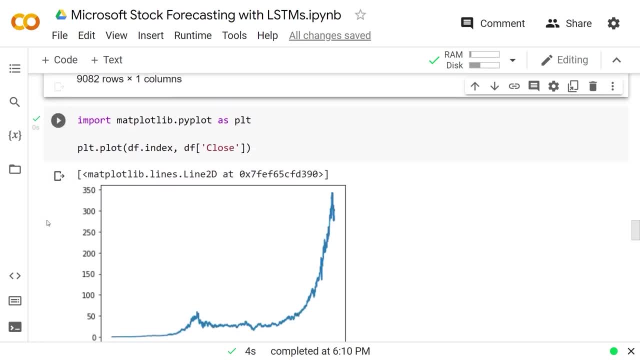 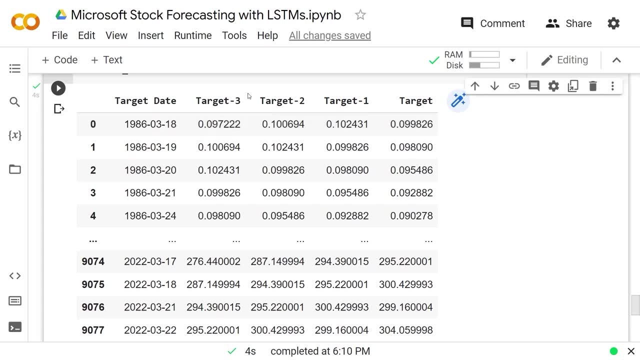 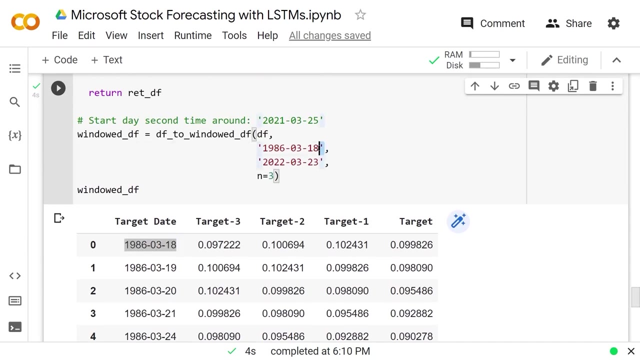 minus one, and this is the target. We have that for every single date that it allows for. So of course, we couldn't have dates previous than this, because we didn't have a whole three values before it. This was the first date that we could start with, hence we actually called that as the starting date. 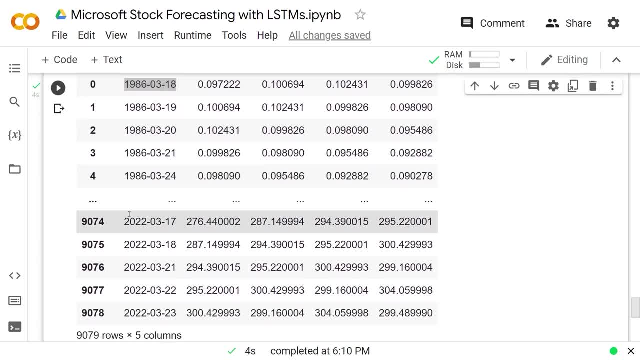 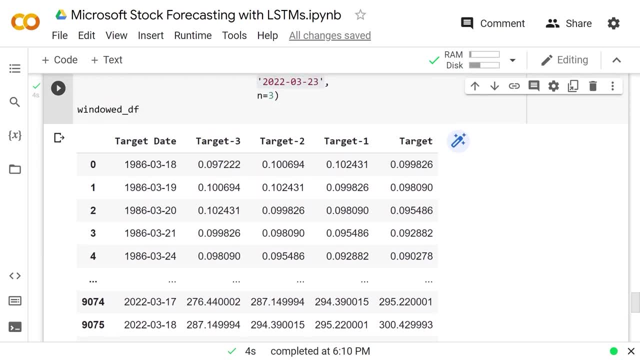 there As the last date. that's the last one we wanted, which is right here, The three previous and then its target value, right there. The reason I started calling it target is to think about this column as the output, because that's what our machine learning model. 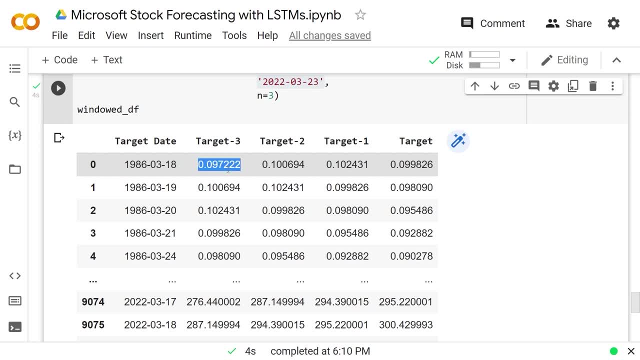 needs. We have what led up to it. so, three days before, two days before, one day before, what is our corresponding output? Because this is the input that's fed into the model and this is the output. It's just like a regression problem or any other supervised learning problem. You have an. 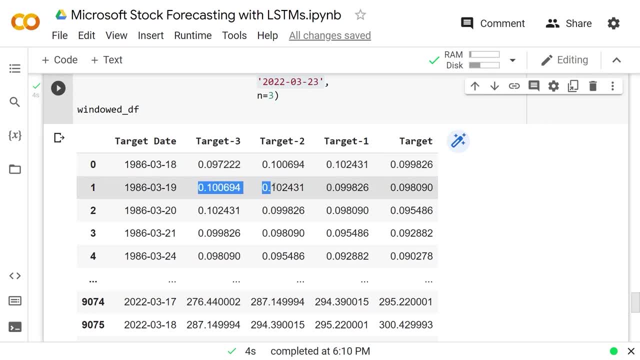 input and then you have an output, and then you have an output. So, if we look at 0.097, and then you have an output, you have another input, you have another output. This is just the whole data frame which displays the inputs, the outputs and the corresponding date for that. 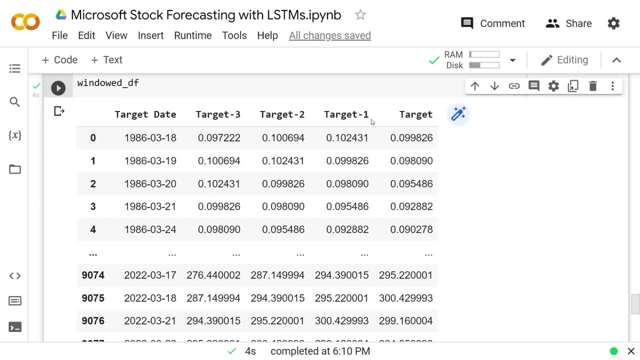 output. So that was really how we converted this problem to a supervised learning problem. We set up its output date with that output and its corresponding input for that row. Now we just need to convert this into numpy arrays so that we can feed it directly into a tensorflow model. 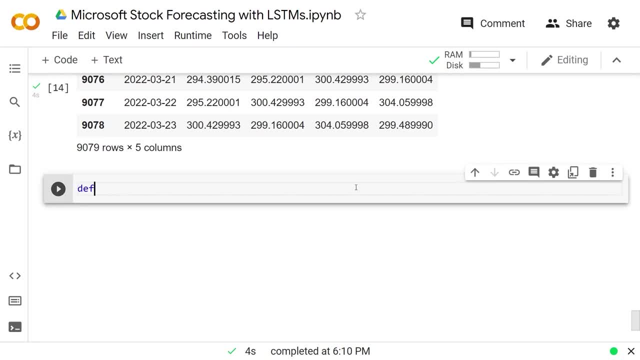 So to do that, we're going to create a model that's going to be called a tensorflow model. So to do that, we're going to create a function. We're going to call it windowedDF. So it takes a windowedDF like above and converts it to dateXY. Okay, so this is actually three things We're. 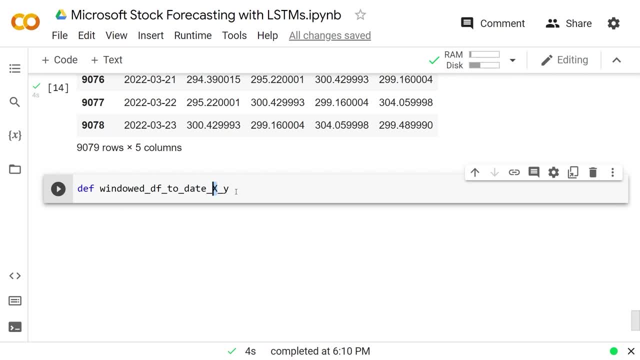 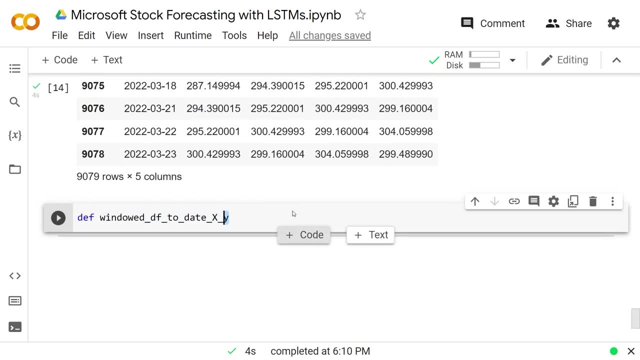 going to get a list of dates. We're going to get an input matrix, X- Actually it's going to be a three-dimensional tensor, We'll see shortly- And Y is going to be the output vector. So X is going to be this matrix here, except it's actually going to be three-dimensional. Y is going to be this: 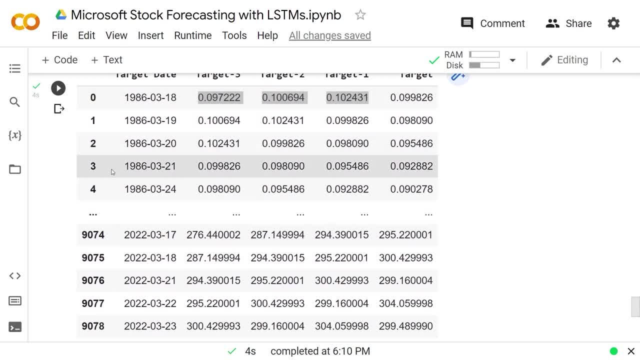 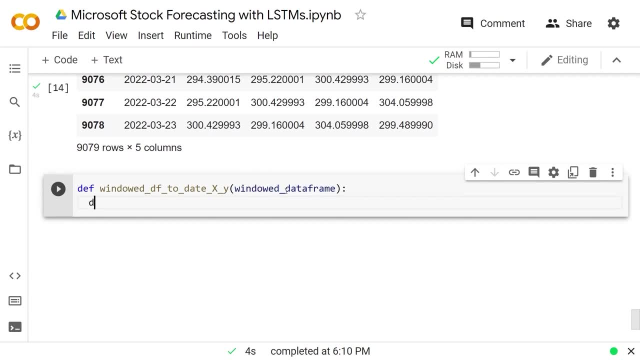 vector here And dates we want to keep those. So dates is going to be this column here. This function is just going to take one parameter called windowedDataFrame. First it's going to do DF as numpy. It's going to convert the whole data frame into a numpy array. We do that with. 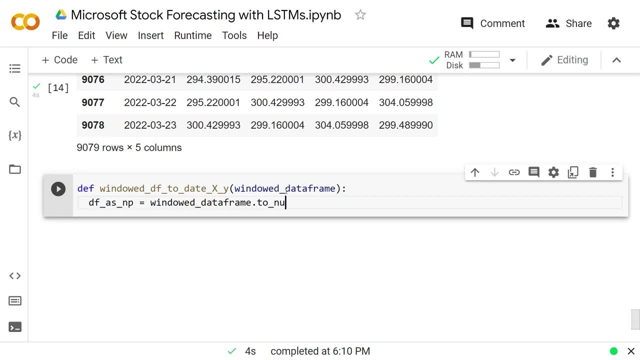 windowedDataFrameto underscore numpy bracket- bracket To get the dates. it's very easy. We just set dates equal to DF underscore as numpy And then we're going to convert the whole data frame And then we need to get all of the rows, So we put a colon And then we put zero, to say just. 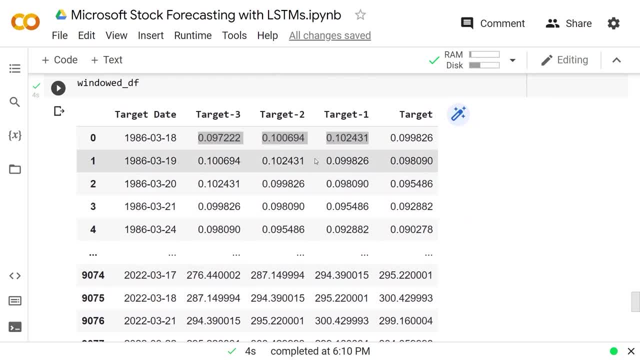 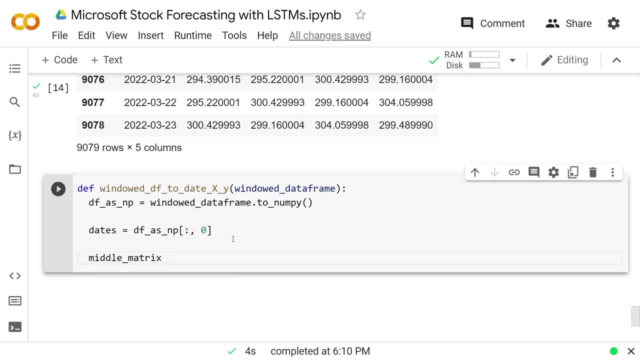 the first column, because it's this column right here. Getting the input matrix is a little bit more confusing, So we're going to call it first middle matrix, not our final input matrix. Middle matrix is equal to DF underscore as numpy. And again we want all the rows, So we'll put a colon. 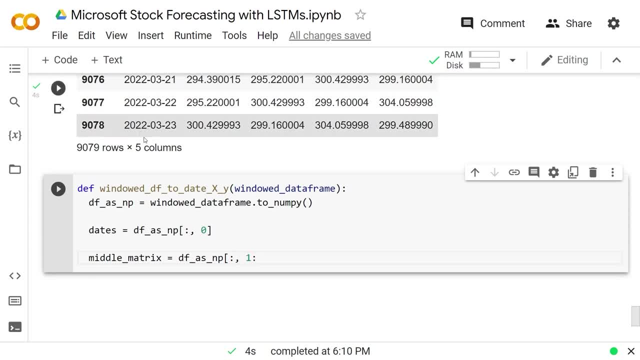 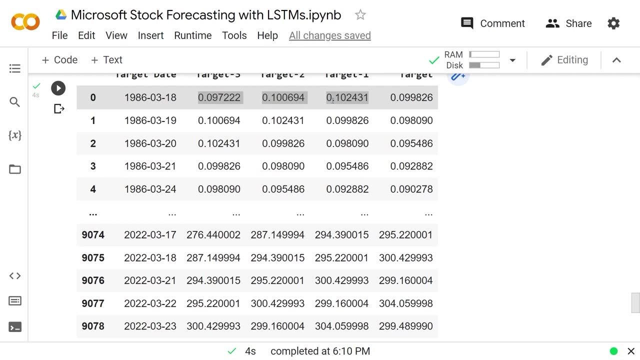 But we only want to start at the first column because we don't want that date column, And then we'll do the last one. So one until negative one says all of these rows here, That's what the colon does, And then the one to negative one says just this piece of information in the middle. So all. 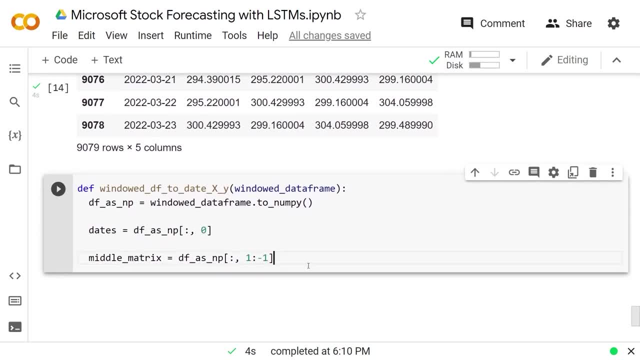 of this piece. Now, unfortunately, what you'll find if you go through like that is that it's actually the wrong shape for the LSTM. We need: x is equal to middle matrix, But then we need to do a reshape. So we'll do a reshape where the first dimension is the length of dates. So this is the. 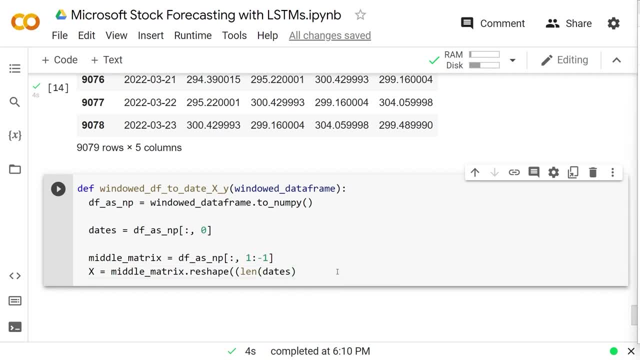 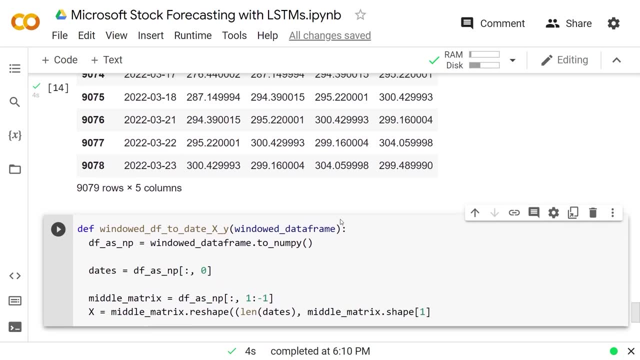 observations. That's pretty common for any tensor flow model. But now we need the second piece of this shape to be middle matrix dot shape sub one. That's just however many columns we had And it would be the same as that n or window value. I'm just making it this because we have access to that. 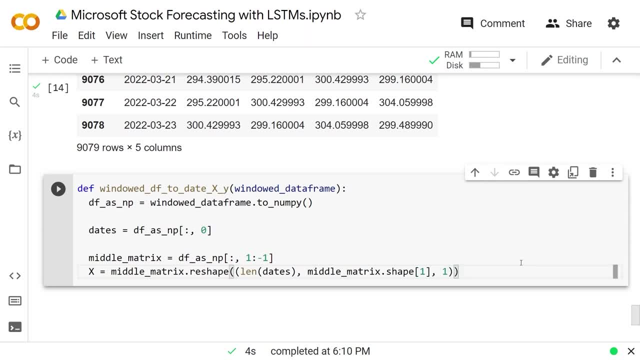 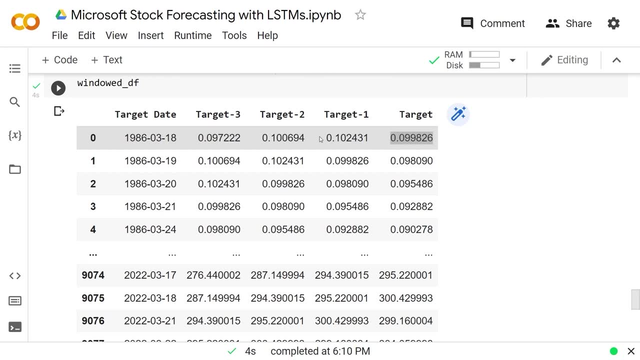 the last piece just has to be a one here, because we're technically only using one variable. we have three different values of that variable and how it changes over time, But we're still only doing what we call univariate for Casting, because we're just looking at how the closing value changes over time. If, instead, we had 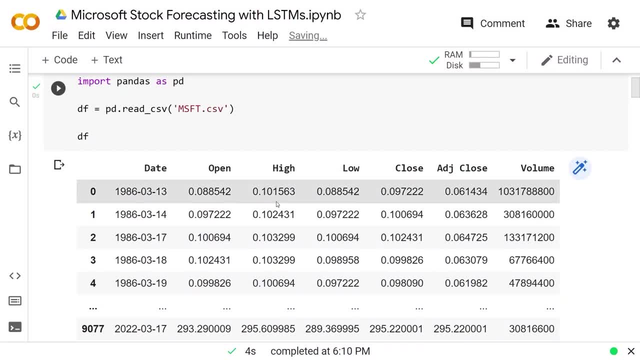 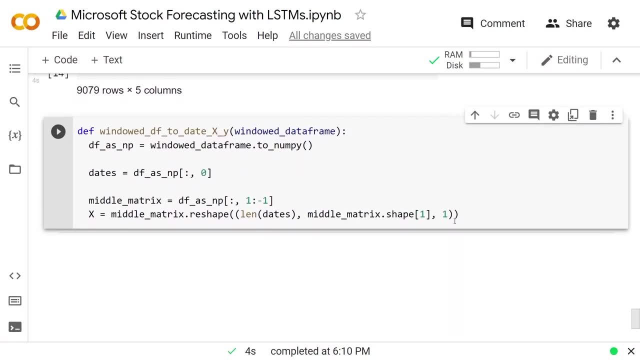 used some of those values at the very beginning, like the open, the high, the volume and those variables. well then we'd have to put a different number down here. we'd have to put two or three or four as this number. we're just doing one because we're doing univariate forecasting Now. luckily, 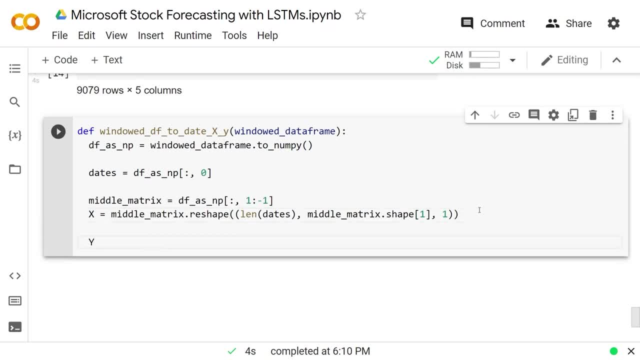 from here. this function is very easy. we can just get our output vector y is equal to df as numpy, not all of the rows, but we only want the last column. that we can just do return three things: dates, x and y. there's just a minor difficulty. if you go on later you'll see that has an error. 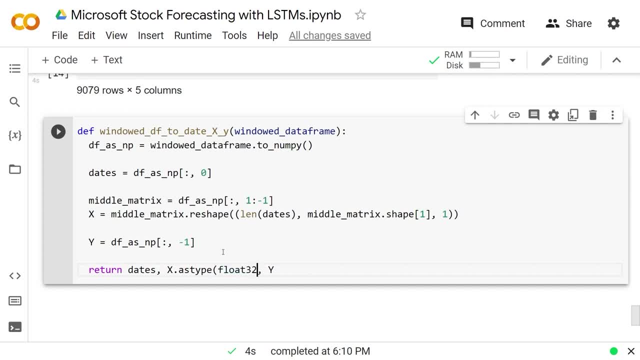 that we can fix with dot as type float 32.. Actually np dot float 32.. If we change those for x and you also do that for y, y dot as type numpy dot float 32, you'll fix a weird error you'll find. later. Now to call this function. we again want the function to be equal to df as numpy dot float 32.. Now to call this function. we again want the function to be equal to df as numpy dot float 32.. Now to call this function. we again want the. 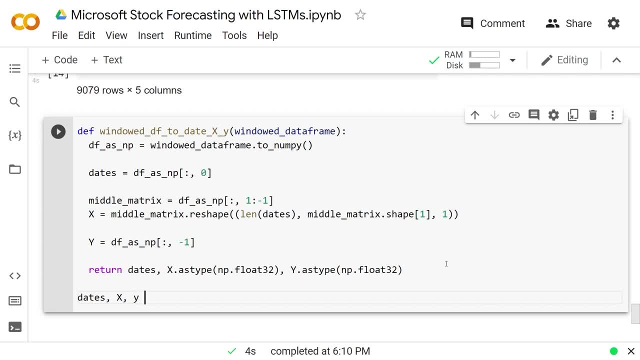 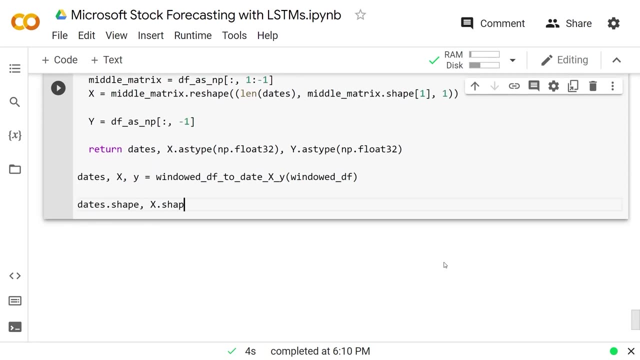 those three things will get dates x and y. set that equal to windowed df to date x, y, just our function there and we'll pass in our window df from before. these three things should be numpy arrays. So we will get dates dot shape- x dot shape and y dot shape and see that we have 9079 of each. 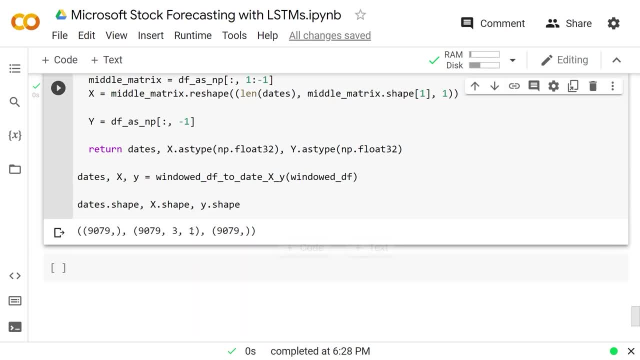 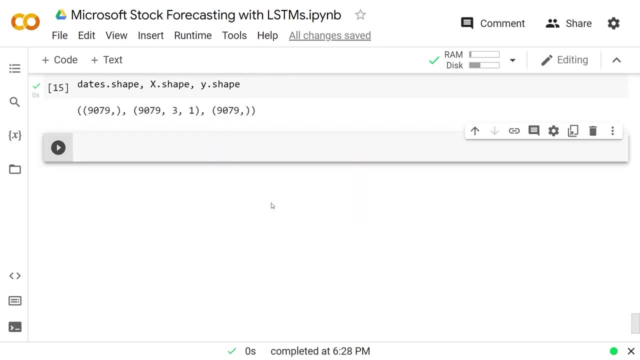 of these three things: our input matrix, and then three by one, because we're looking three steps in the past, but for only one type of variable. Now we're going to split the data into train, validation and testing partitions. The training will train the model, the validation will help train the model. 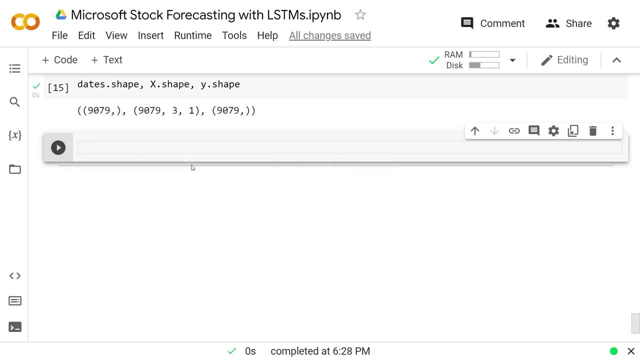 and then the testing is what we're going to use to really evaluate the performance of the model. We need two integers to help with the split. We'll get q80 first. That's going to be the integer of the length of dates times 0.8.. 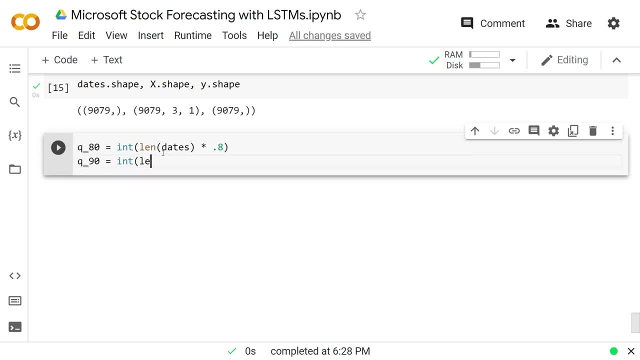 Then we'll get q90, which is equal to the int of the length of dates times 0.9.. So we'll make the training partition, the first 80%. so we'll get dates train, x train and y train. Each of those are going to be each of their pieces. 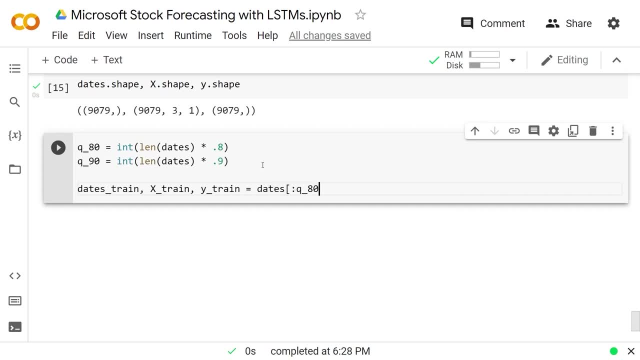 so this will be dates, but then only up until q80 to make it the first 80%. We'll do the same thing with x. so x up until q80, and then y up until q80.. Because it's a little bit slow, I'm just going to paste in these two lines to get val and test. 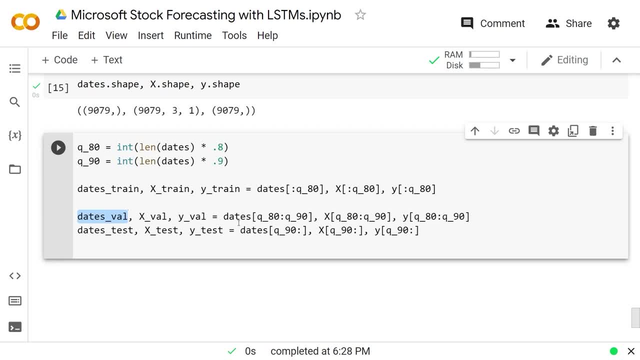 which we can get val dates, val, x val and y val by going dates q80 to q90, then x, q80 to q90, and y, q80 to q90.. That's all that information between the 80% and 90% pieces. 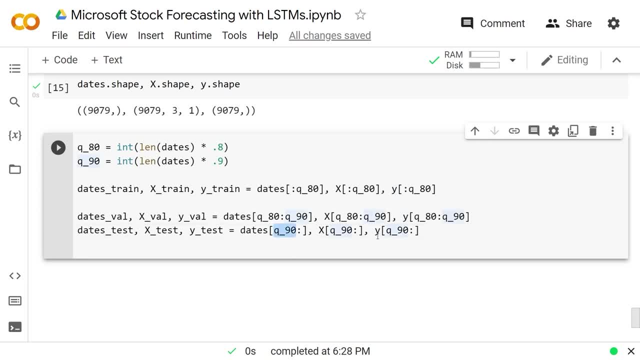 Then we just get the testing information by saying q90 onward to get that last 10%. So you can see it's ordered. The first training piece is up until the first 80%. The validation is the 80% to 90% 10%. 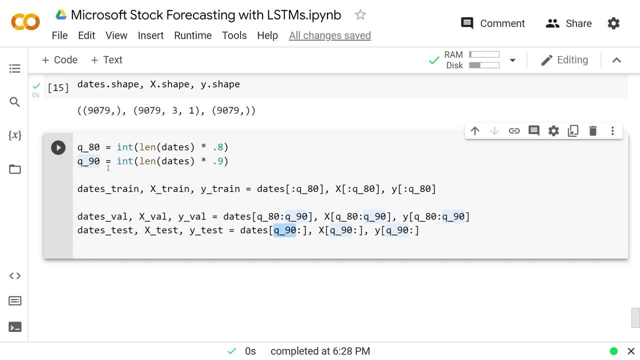 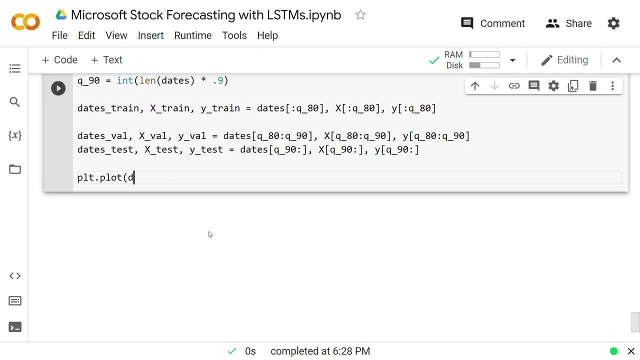 and then the test is that final 10% from the 90%. We can visualize and color this very well with matplotlib, so we'll do pltplot, then we're going to get dates train and then y train. We'll do the same. so pltplot for val, so dates, underscore, val and y val. 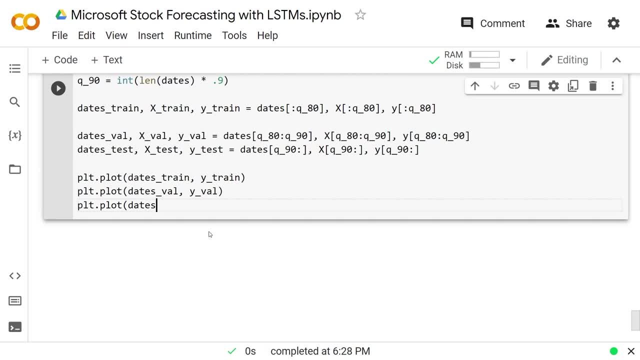 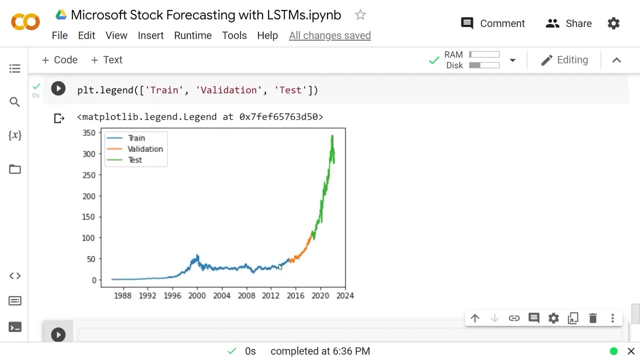 Finally, the same for test: pltplot dates, test and y test. and we'll just add in a legend so that you can see which is which, although it should be pretty obvious: pltlegend train, then validation, then test. if you plot that you're going to see that train. is all this information here. 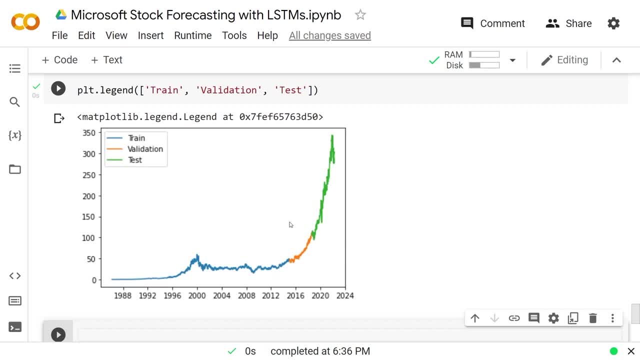 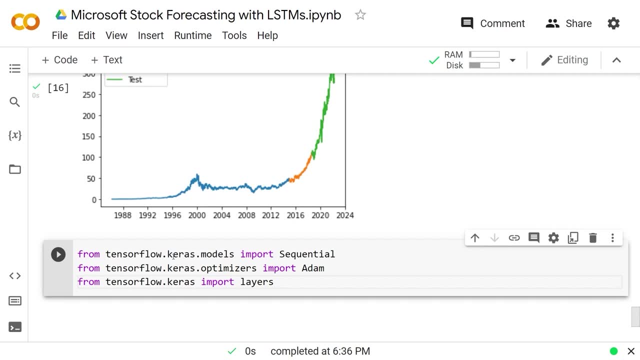 marked by the blue. then validation: is this piece? and then test: is this piece? here It's time to create and train our model. We can do a few imports from TensorFlow, From TensorFlowcuresmodels, get sequential. We're going to build a sequential model. 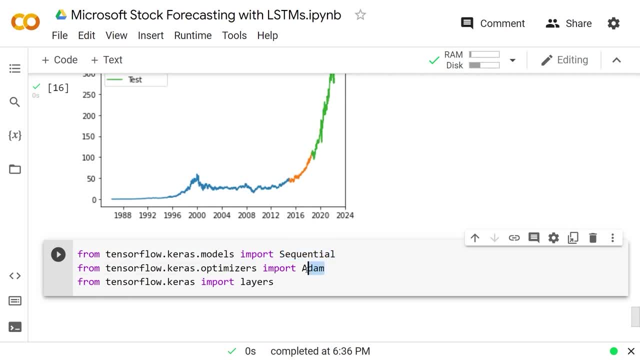 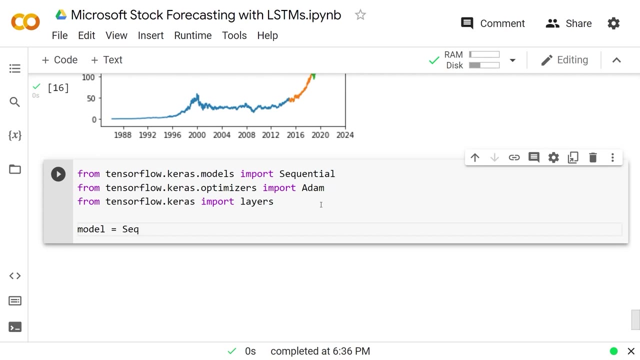 From TensorFlowcuresoptimizers we'll get atom. That's the optimizer we're going to use. And then from TensorFlowcuresimportlayers we'll make a model that is sequential and built up of many layers. So we'll define our model and we're going to call it model is equal to a sequential. 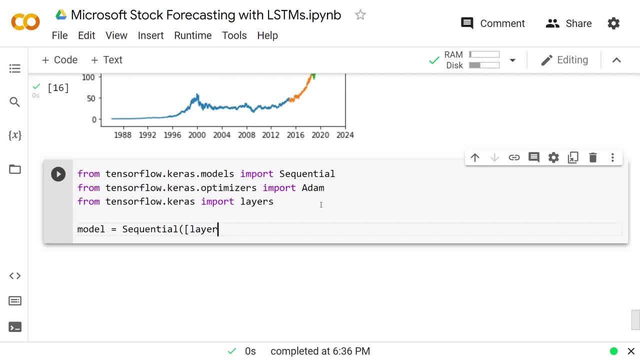 and then we'll pass that a list of layers. So the first one is just the input layersinput, and we need to specify the shape of the input. Remember, we don't need to specify the batch number or how many examples: 3 by 1.. 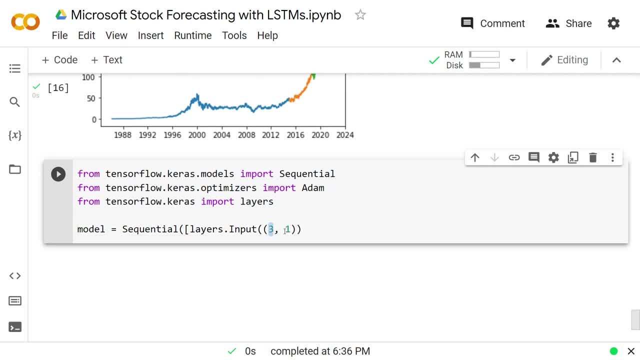 Again, it's 3 because we're doing 3 days in the past and then it's 1 because we need only one feature, only univariate forecasting. Now that we've specified the input layer, we're ready to do an LSTM layer. 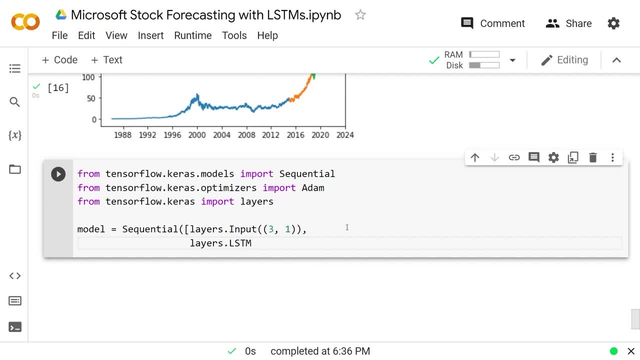 So we will do layersLSTM, and this number is relatively arbitrary, but we will choose 64, which is a relatively big, but not super big number of neurons for the LSTM. All that you really need to know about this number is: the bigger the number. 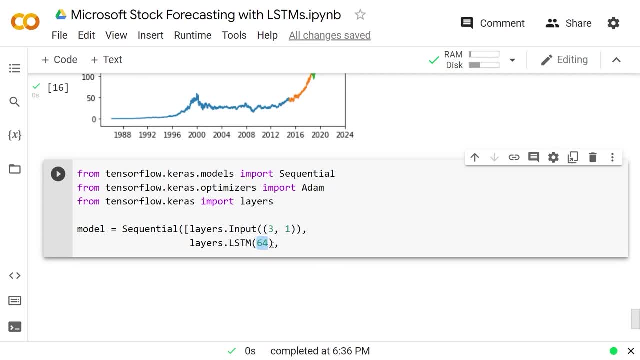 the more complicated the model is, the more prone it is to overfitting and the more heavy duty it is considered. We will add, instead of an LSTM, a number: LSTM, a dense layer, layersdense. we'll choose 32, for a similar reason as above. 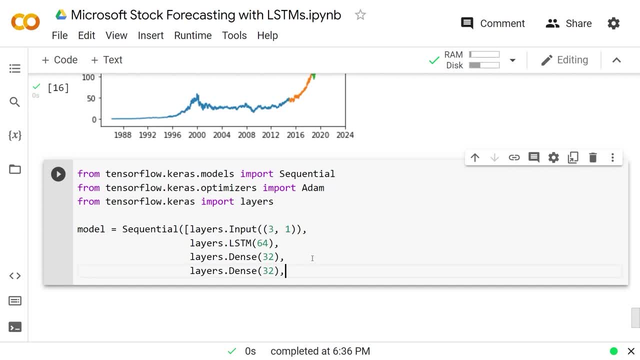 You're also very welcome to stack dense layers, and so we'll just actually paste that in again and have another 32.. We're not going to mess with the activation functions for the LSTM, but for the dense it's usually a good idea to set activation equal to ReLU. 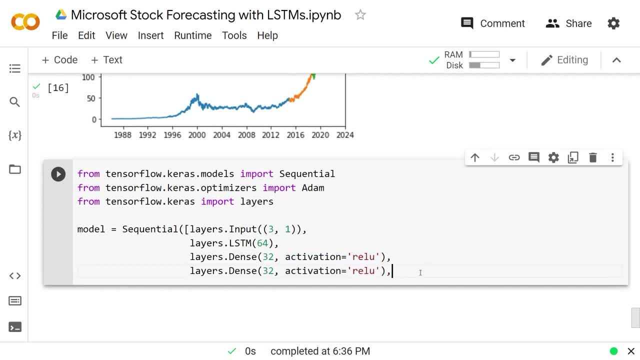 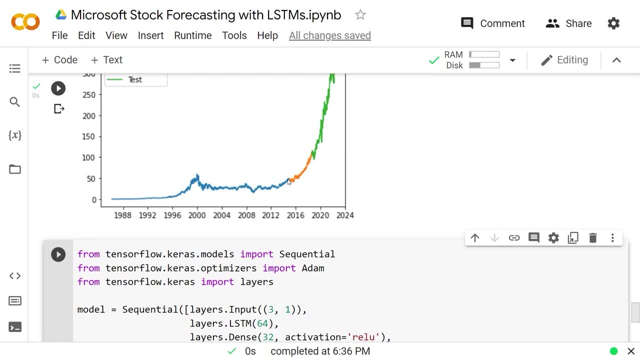 So we will do that for both of those dense layers. Now we must specify the output of our model and since we are only forecasting 1, we're just trying to predict, say, the next value. we only want this to be a layersdense of 1,. 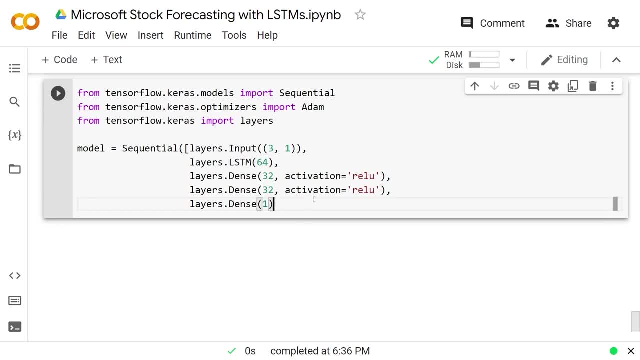 where we don't change the activation function as by default, it's linear which is desired. We can now close this up and specify that the model is going to be compiled. To compile the model, we must set the loss function, and the loss function we want to minimize is the mean squared error. 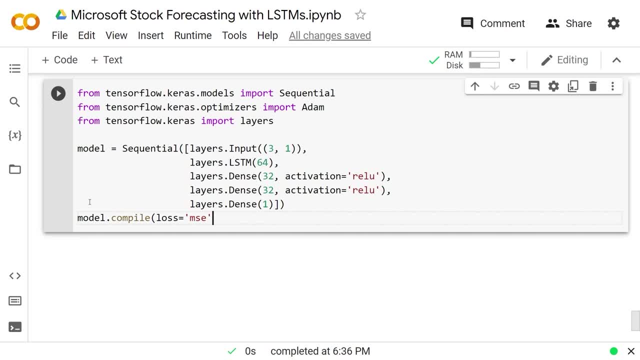 so we will just write the string of MSE for mean squared error. We also need to specify that the learning rate is going to be equal to the optimizer. So we will set the optimizer equal to the atom optimizer, where we specify that the learning rate is equal to. 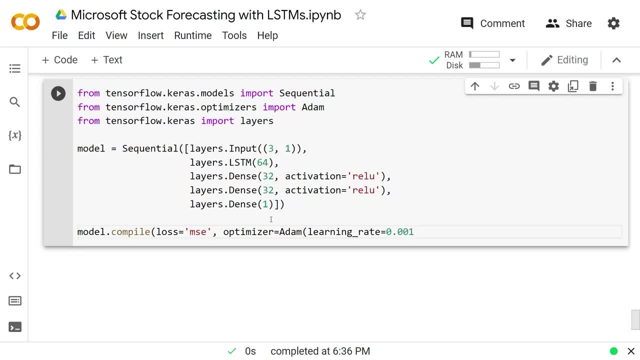 for this example, it turns out that 0.001 is going to work out pretty well. If you're doing a different problem, the learning rate is something you definitely want to play around with. as well as these values, here, We also want to specify a new metric. 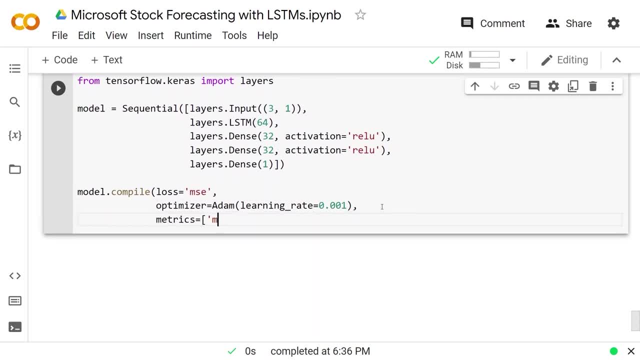 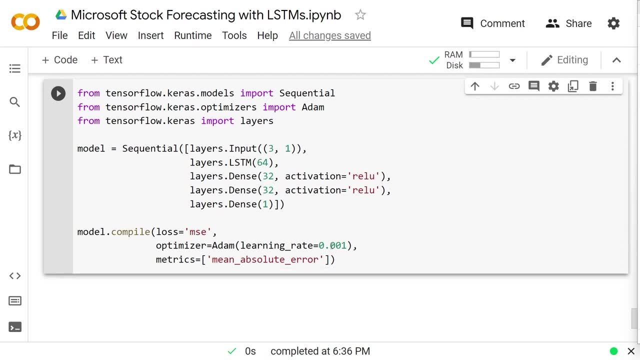 it's going to be metrics equals. we need to put it in a list. it's the mean absolute error. This number tells us on average how much we're off by, rather than the squared distance. We'd rather look at this. although we need to minimize the MSE. 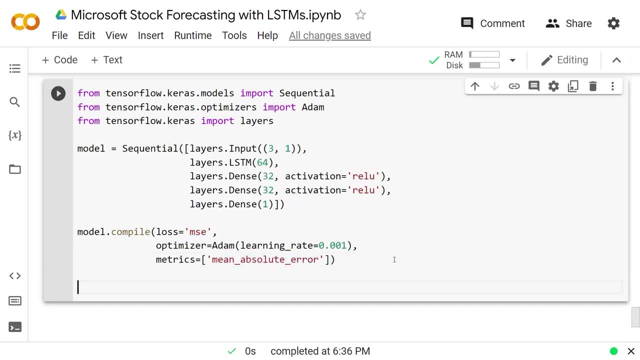 as this is not differentiable, We're now ready to fit the model so we can do modelfit. we pass our inputs of xtrain and ytrain and then we specify that the validation data is equal to the tuple of xval and yval. 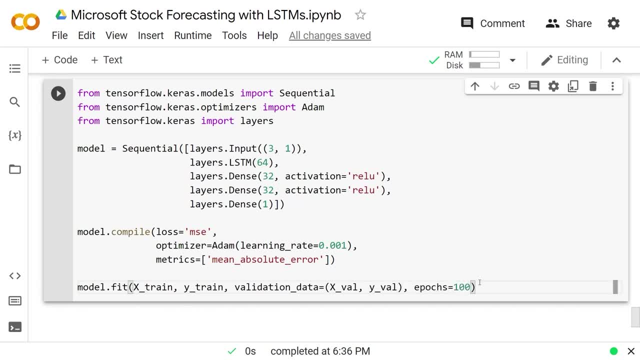 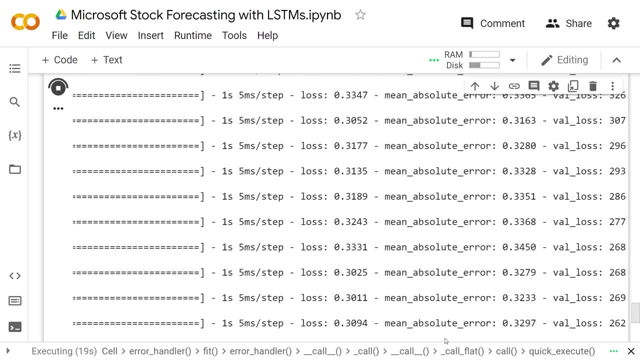 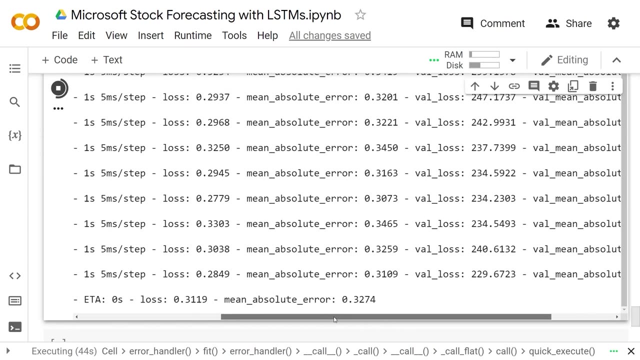 We're going to let this run for 100 epochs, which means 100 runs through the dataset. I'm going to press enter and we can see what happens. As we can see, at this point it looks like it's not really changed very much. 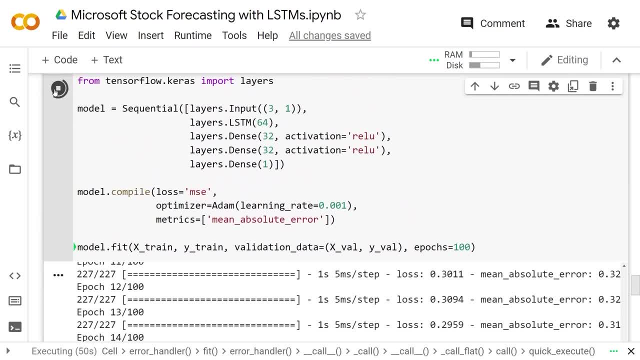 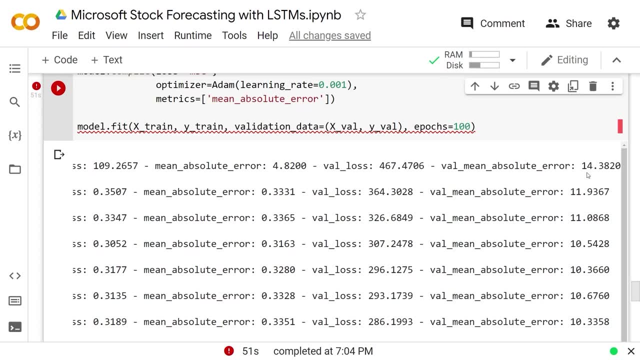 so we can actually cancel this and it is going to save whatever progress it's done so far. Now to briefly analyze this. we mostly care about the validation mean absolute error going down. We can see it's at 14 at the beginning. 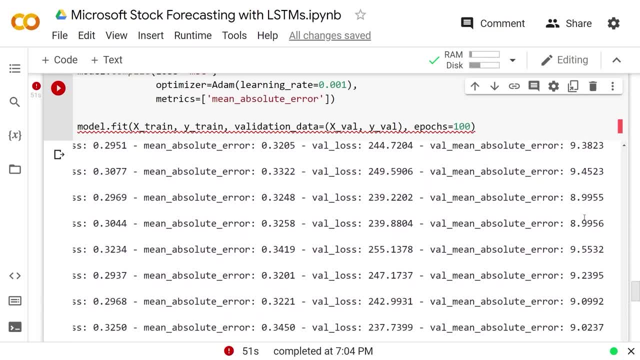 then it goes to 11,, 10,, 10,, 11,, 10,, 9, and then it hovers around 8,, 9,, 10, and that's when I was ready to stop it, because it wasn't really changing all that much. 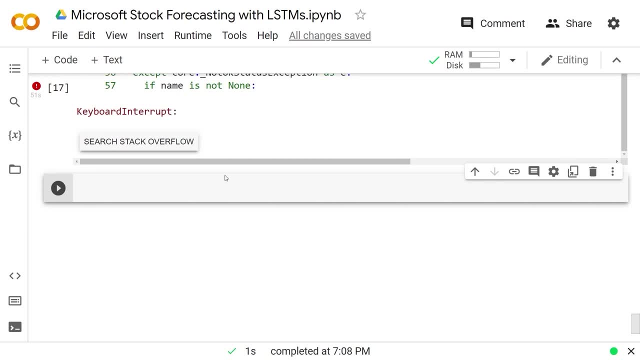 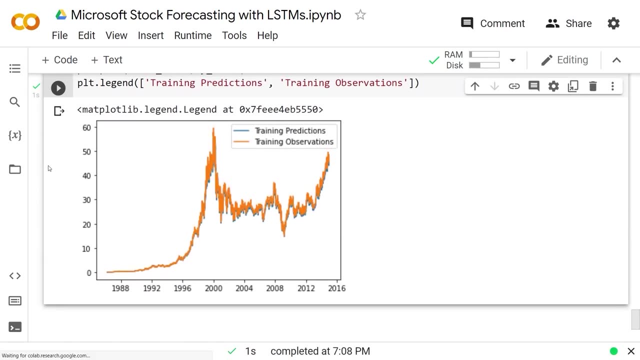 It's much easier to visualize what's going on instead with graphs. So before worrying about the code, I'm just going to show you the pretty picture we can make for it. predicting on the training set. So the orange is the actual observed observations. 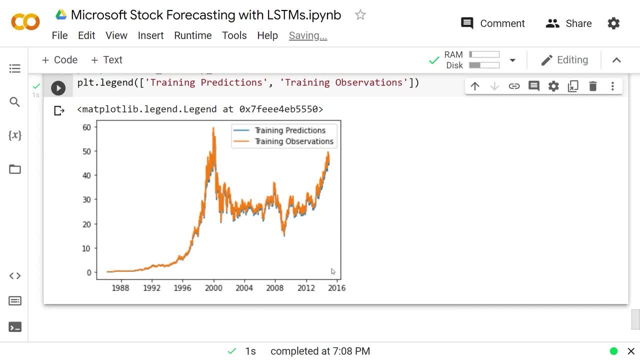 it's what really happened from 1986 to 2016.. The blue is what we predicted, So each time it got the three previous and it tried to predict the next one. That's also what it was trained on To make that run. 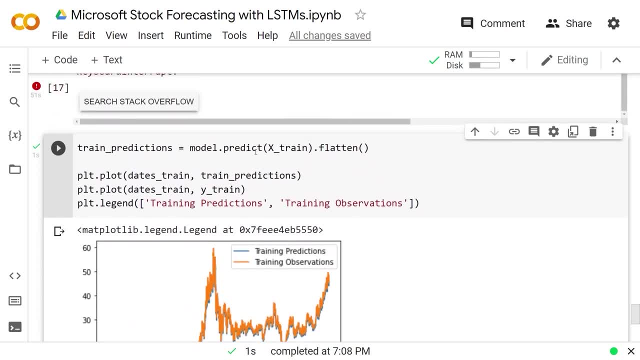 we simply get the training predictions with model dot predict on x train and then we have to do a flatten. Then we can do a plot of dates train and the train predictions and dates train and y train. That's that blue and the orange curve. 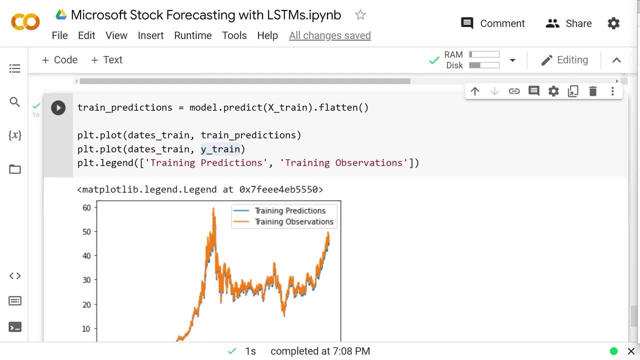 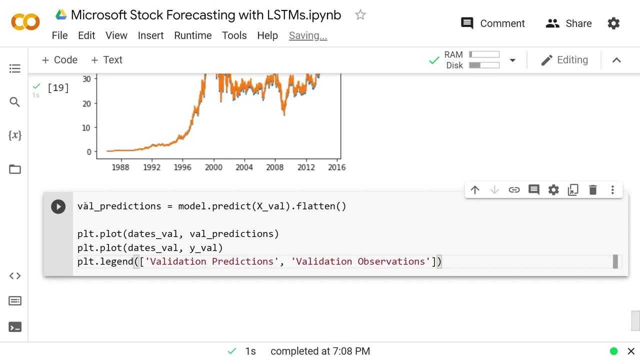 And then we just create the legend. Since I explained that code for the train, I feel no real need to explain it much. for the validation, as this is literally the same thing, but replacing the word train with val. So for the validation. 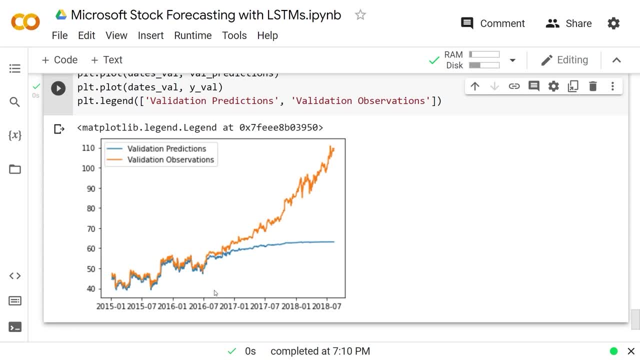 we get this graph where it follows it until you know about 2017, and then it just really flattens off, which is the same time when it actually starts to pick up. So the observations: what really happened is it went up like this: 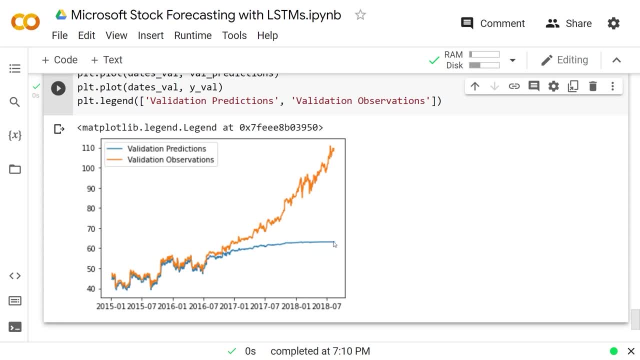 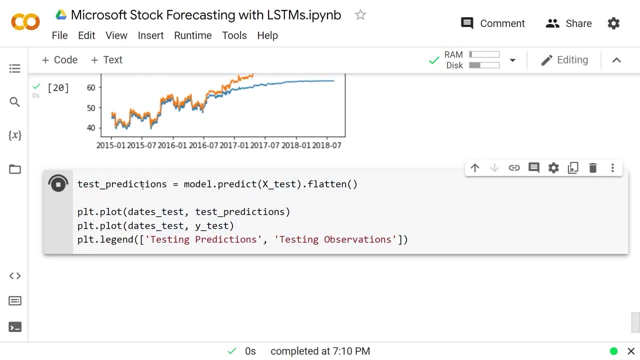 but the predictions. it actually just started to zone off and it couldn't follow it anymore If we were to look at the test. this is again just replacing that word train with test. This picture is even worse. It doesn't follow it at all. 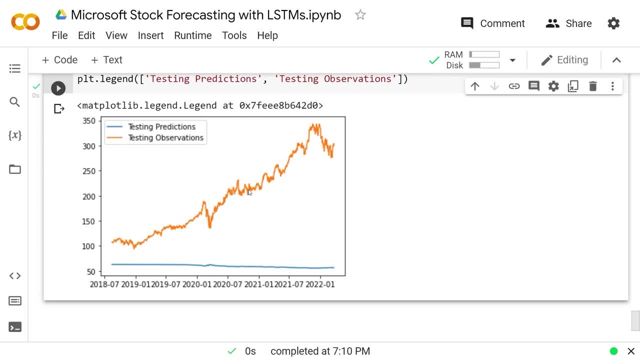 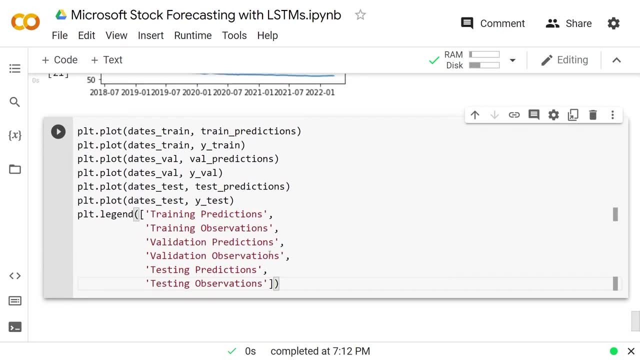 It actually thinks it's going down a little bit, whereas it's going up a lot, and then it goes down. I'm now going to put all three of those pictures on the same graph Again. the code is not hard, it's just annoying. 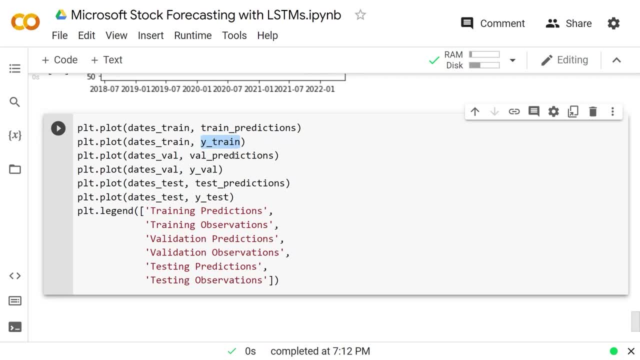 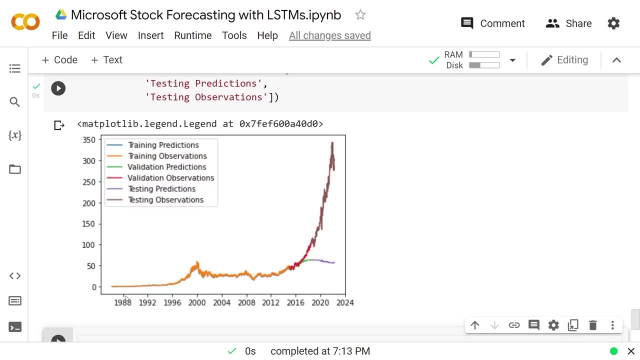 where we first plot the training predictions and the observations, the validation predictions and the observations same for the test, and then we create the legend. We see that this picture again for the training, it follows it very closely and for the red piece. 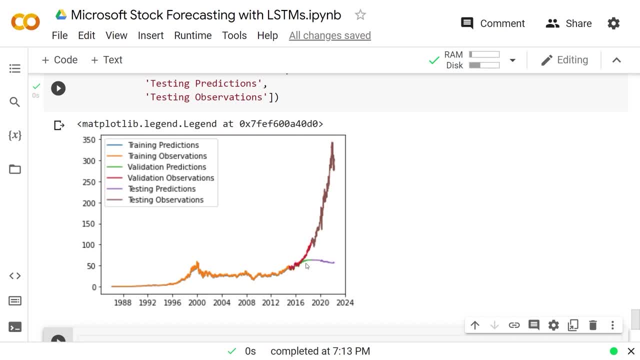 is what actually happened in validation. the green is what it thought happened- Not good at all. The brown is what really happened and the purple is what it thought for the test- Really really bad. at that point It turns out that these LSTM models are very bad. 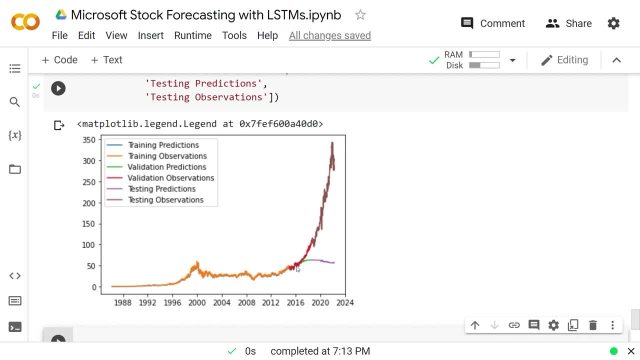 at what we call extrapolating, and so if it was trained on data only in this range here, only up until like the 50 value, it's not going to be good at predicting stuff this high, Even though it is given, say, as input, these three values here. 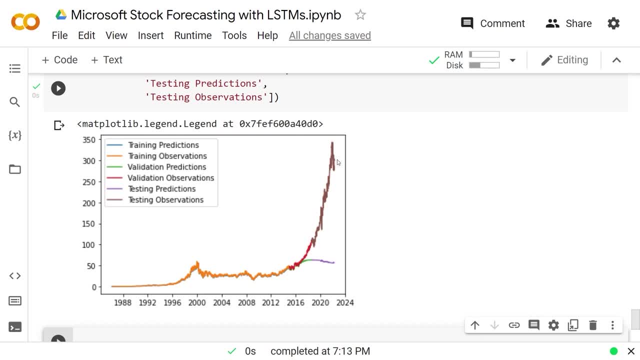 it has no idea what to do with them because it's not going to extrapolate well. Extrapolate means basically learn data outside its range. A line extrapolates well because if we drew a line here, we could just continue drawing that line up like that. 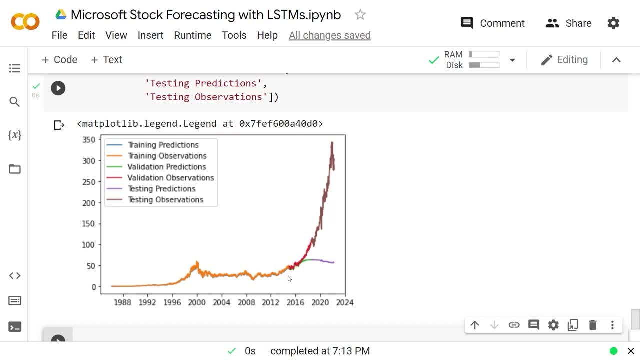 But if the LSTM is only trained on this data here, it will have no idea what to do when the values are increasing and are this big. Another way to think about it is that all this information here, it might actually not be that helpful. 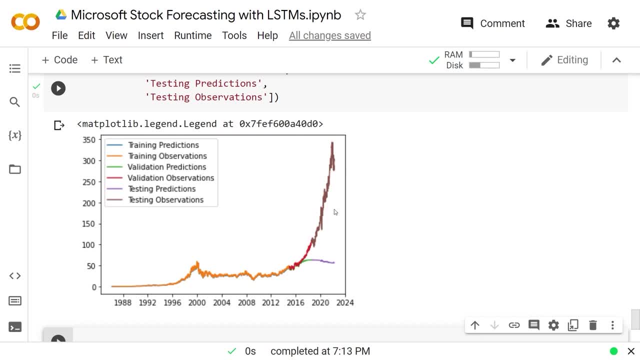 Because over here the values are way up like this and the pattern starts changing a lot. So maybe we don't want to train it on all of this, maybe we just want to train it on, say, this information here and then validate over here. 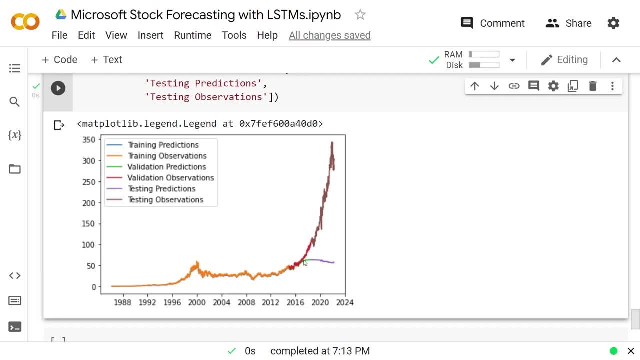 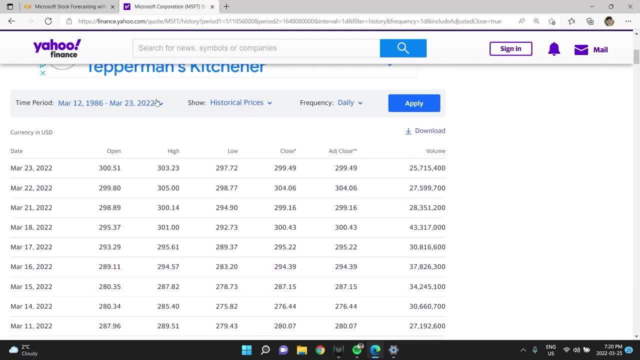 So we'll do just that. We're going to pick some day over here to start training at. We do need to know that this date is actually in the dataset, and for that we'll go to our dataset over here and select the time period of one year. 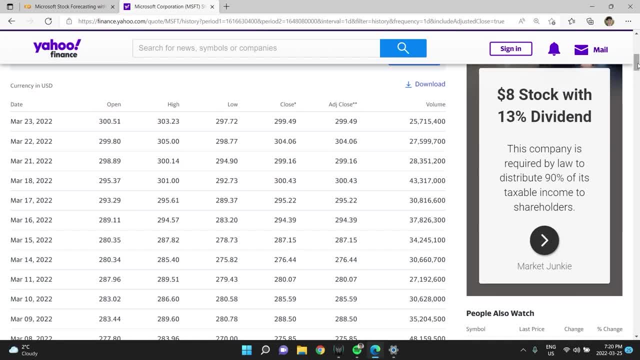 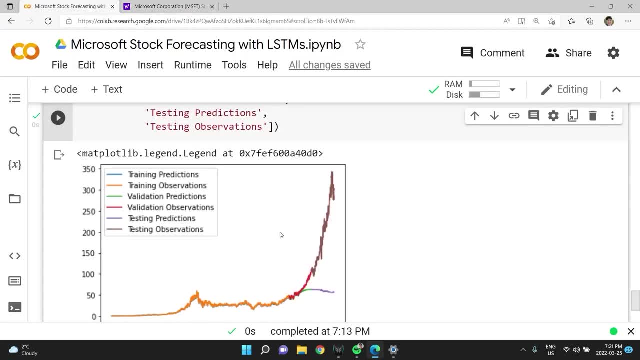 And if we apply that, we just need to scroll back all the way to the bottom and see that one date that we know exists is March 25th 2021.. We will use that as our starting value instead. So that means we need to change our windowed function above. 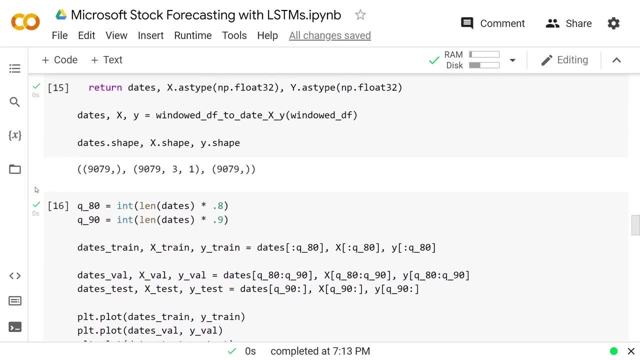 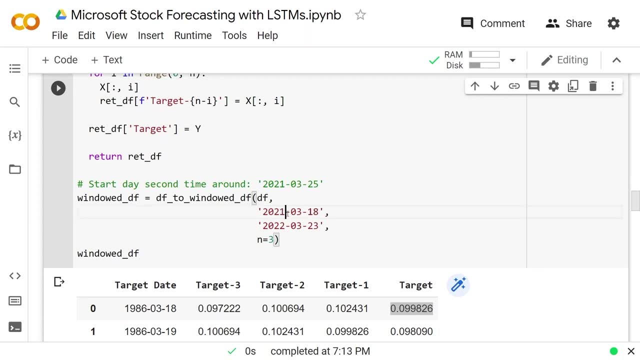 Or not actually change the windowed function itself, but just change how we're calling it. We need to change this value here to be, the year is going to be 2021,, 03 is fine and then 25 is the date we know exists. 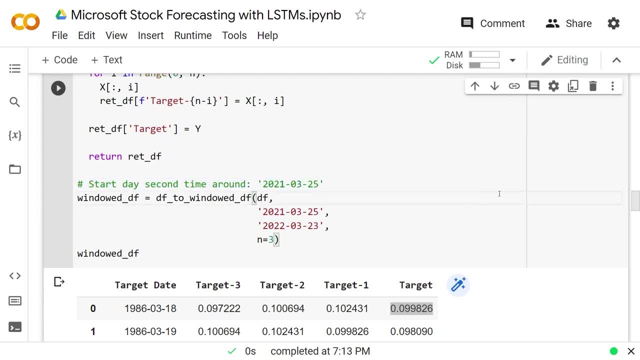 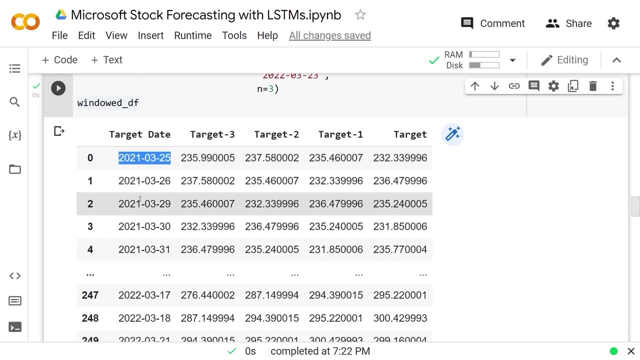 As you can see here, I had this in a comment for me to remember, So now the first date will be 2021, 0325,. and these are its corresponding information. The end date is exactly the same and we only have 252 rows this time. 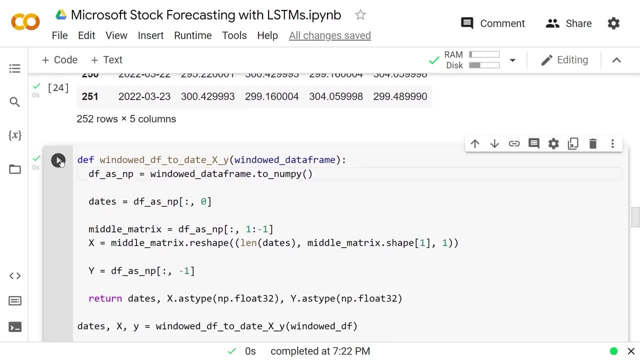 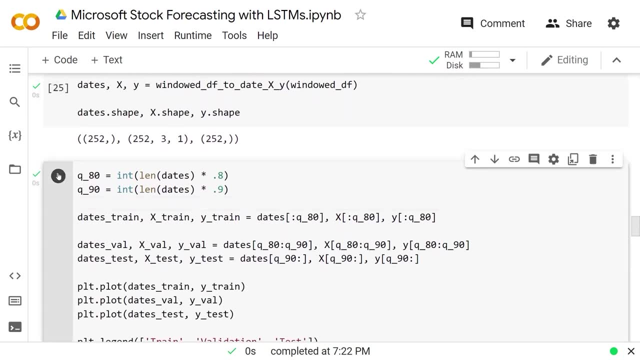 way less information. We should have no problem just re-running the cells we already did, so we're going to do that which gets dates x and y. Note that they're smaller. this time We'll again split the dataset and make sure that we plot it properly. 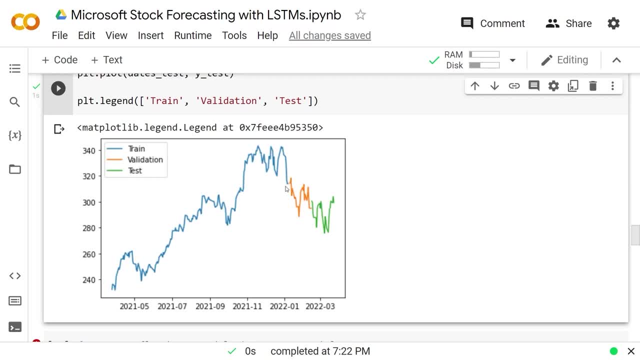 So our starting date up until about the middle over here is train, then validation, then test and note that we've already seen values in this range, so it should be okay to predict values in this same range over here, Since we only changed the number of things the model's seeing. 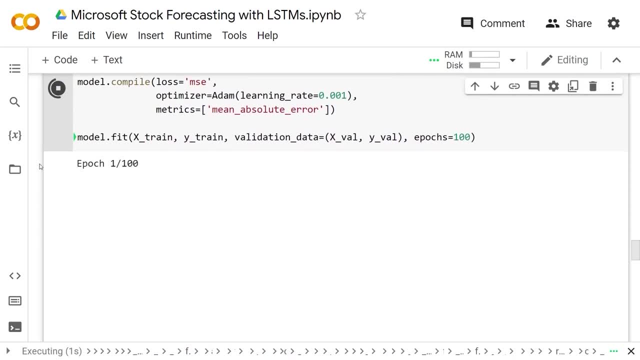 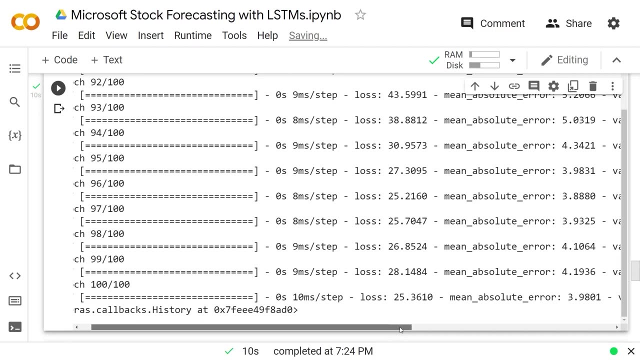 the model is actually fine as is. We can run that again and it's going to run a lot faster. now We'll see again that our mean absolute error goes down pretty low and for the validation a lot better than it was before. 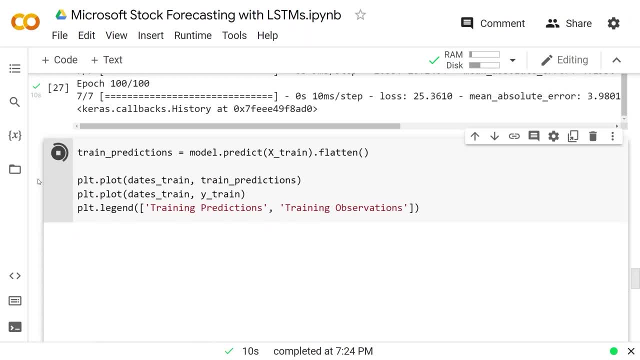 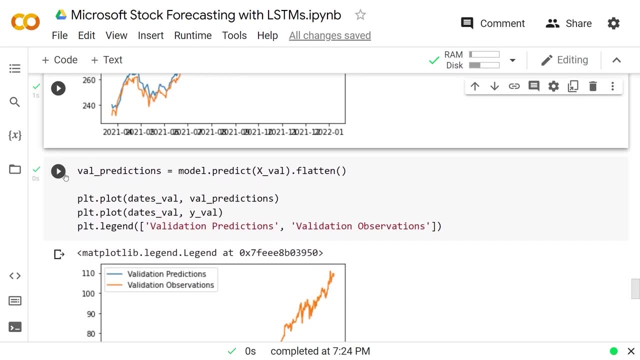 We can recreate all of our graphs so to plot the training, we can see here the train. It doesn't follow it quite as well as before but that's totally okay If we see here for the validation. it got so much better. 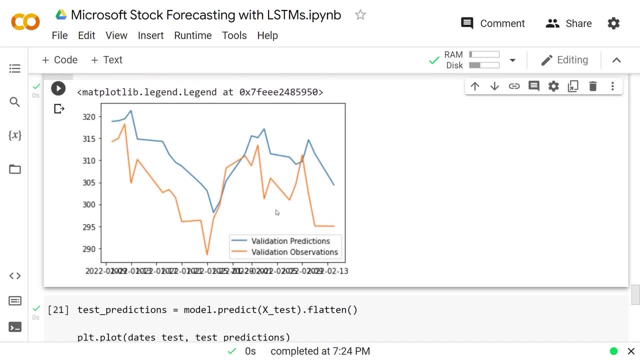 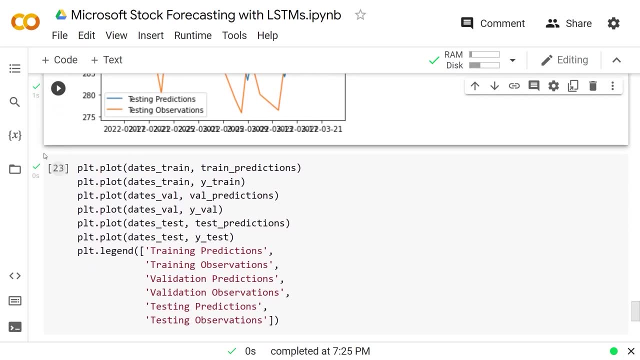 Now look at how zoomed in this is. These values are extremely close to each other, And if we were to do it for the test as well, the tests are also extremely close to each other If we were to plot them all on the same graph again. 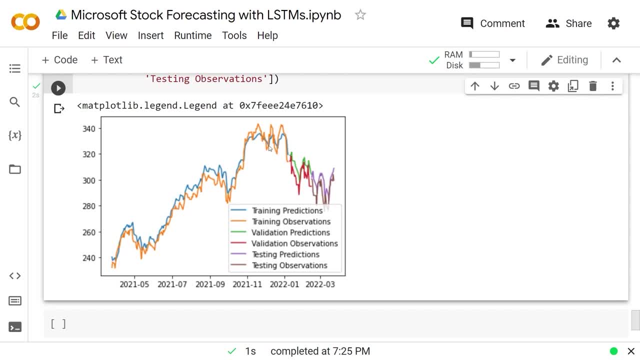 we would see here, zoomed out, that they're all very close to each other. So the predicted first, the observation is very, very close, no matter whether it's the train, the validation or the test. Now the video could be done here. 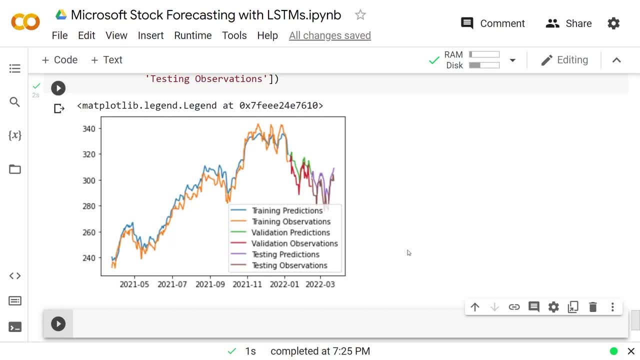 but I want to show you how you could try and predict long term, Because all of these values, any of these predictions, we're assuming we had the actual three days before and that data was real, then we used those three days before to make the prediction. 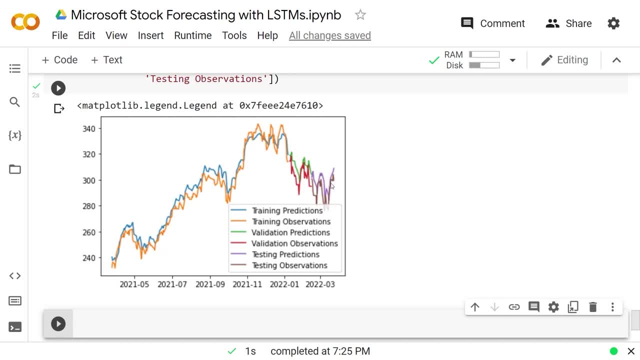 And then the next day we would have the actual three and then we'd use that to predict the next day. Well, what we're actually going to do is train here and then pretend that's all the data that we have and let the model recursively predict the future. 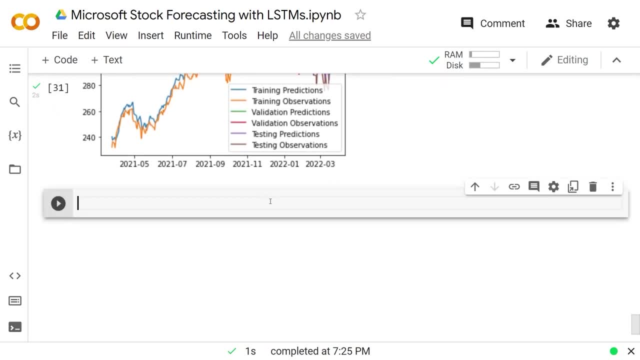 and see what it has to say. So to make that function, we're first going to do from copy import deep copy. We'll make a list and start to build this up, called recursive predictions, is equal to an empty list. 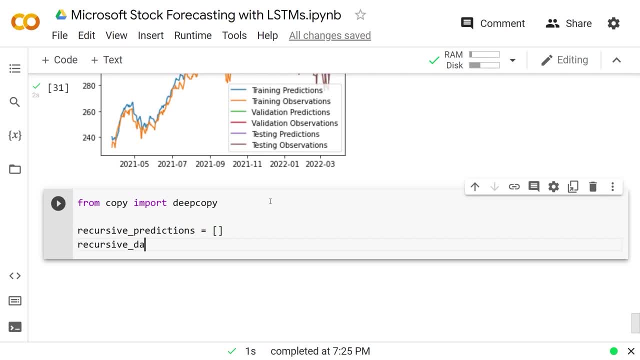 And then we'll get recursive dates. these are the dates on which we're predicting, for This is already known, and this is equal to npconcatenate the dates val and the test val. This is because the dates we're predicting 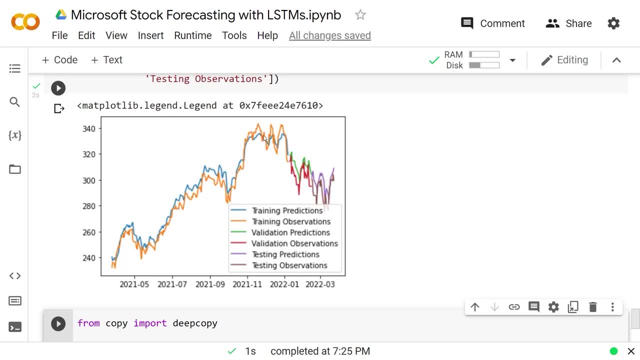 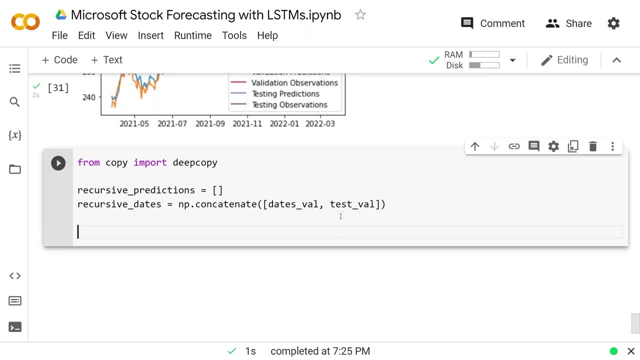 are here onward. So we're training on all of this- in fact we've already trained on all of that- and then the recursive predictions are going to be for these following dates. So now we can loop through those dates for target date. 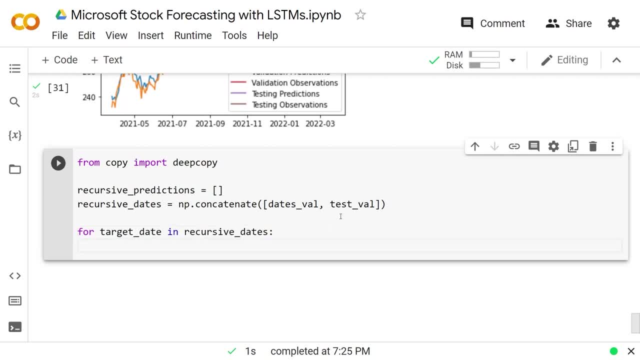 in the recursive dates we'll get our most recent input. So the last. we'll call it window. I'm just copying it so we don't change anything. deep copy of xtrain sub-1.. Because the last window that we actually had access to, 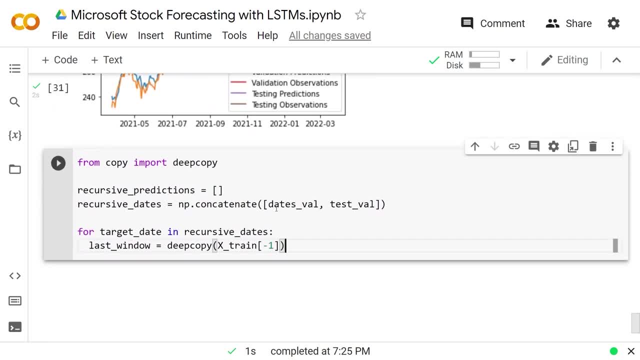 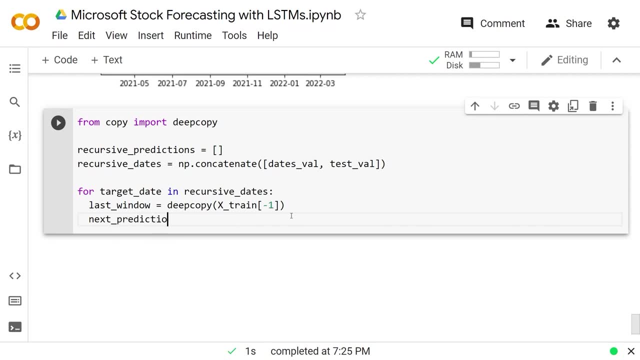 was the very last 3, over here That is stored in xtrain sub-1, and we need to start predicting for the future, So we need to get our next prediction. so the prediction for the next day that will be equal to. 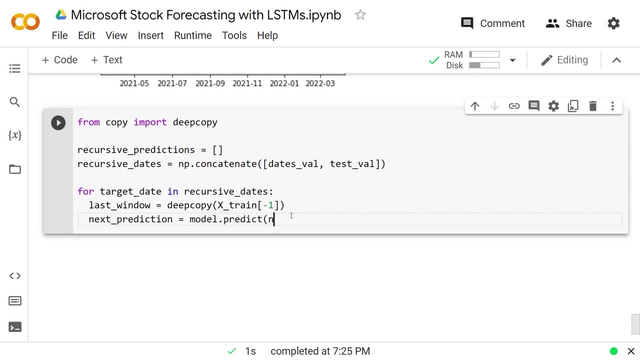 modelpredict. unfortunately we actually have to make it the numpyarray of the list of the last window, but really it's just the last window. don't worry too much about that piece. That and then flatten it like before. 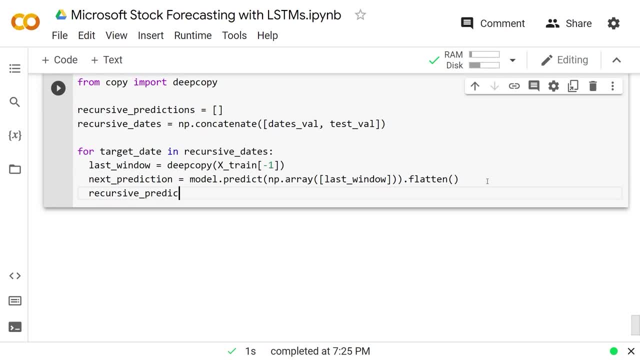 Then what we can do is recursive predictions, dot append. So add that to our list with next prediction. Then we need to update this last window, Because we just made a prediction for the next day. well, now we need to move on. 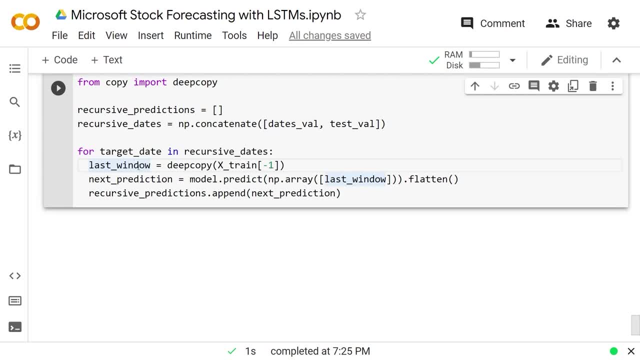 to the previous two informations that were actually seen and then the next predicted value, Because we need to start using the values that we're predicting. that's why it's called recursive predicting. So we'll actually set last window sub negative one. 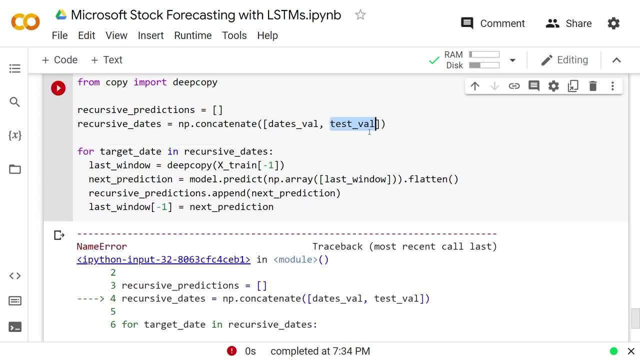 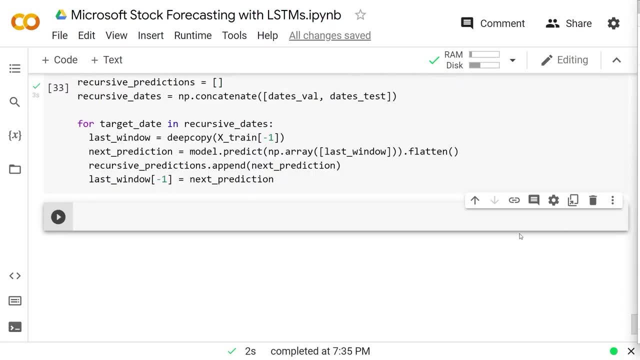 equal to next prediction. Sorry, I have an error here. this should actually be dates test. And then, if we run that, I'm now gonna paste in again some annoying code, but it'll look very familiar. It's exactly the same as that big graph as before. 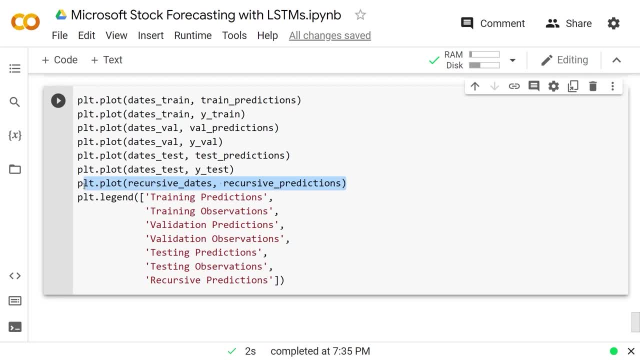 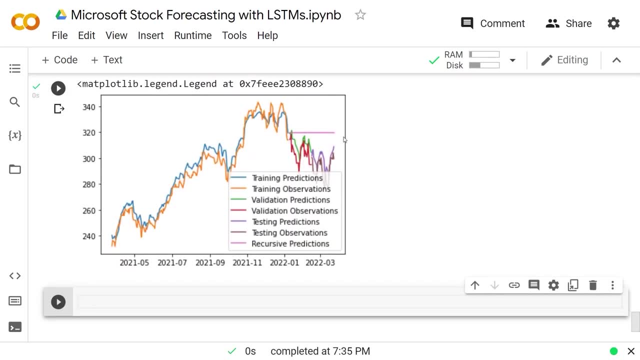 except I added in the recursive dates and the recursive predictions and I put that in the legend as well. If I were to plot this, you will see something very funny. This piece right here is the recursive predictions. The model has absolutely no idea. 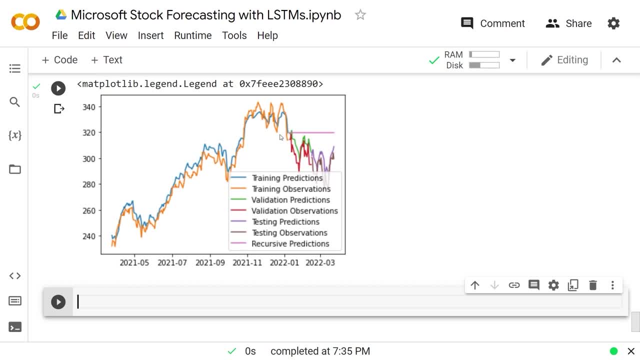 on how to predict in the future. It just thinks it'll be what it was before, and actually that's a reasonable prediction. Predicting stocks is incredibly difficult. There is, of course, the trend we can analyze. we saw before that the graph really started to go up. 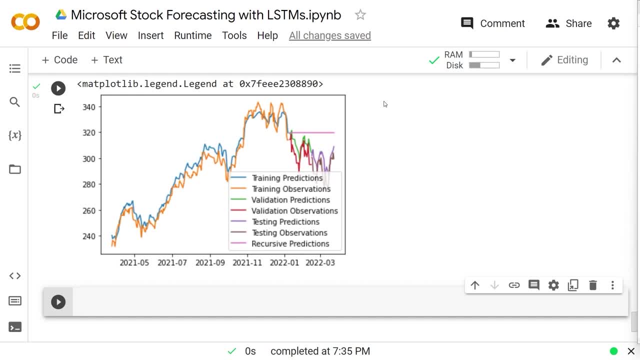 and that would indicate to you that it's a good stock to buy. But that doesn't mean I can guarantee that and I don't want to be liable for you predicting any sort of stocks with any sort of model, And by no means. 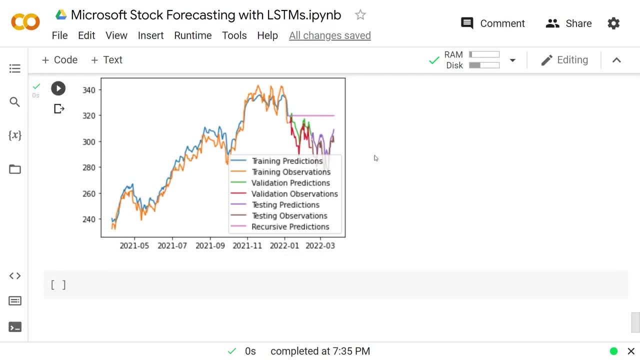 is the model we made useless. It's just on the micro scale of per day. should I sell or buy? Of course, in general, people generally think of stocks for the long term. what should I do to make money in the long term? 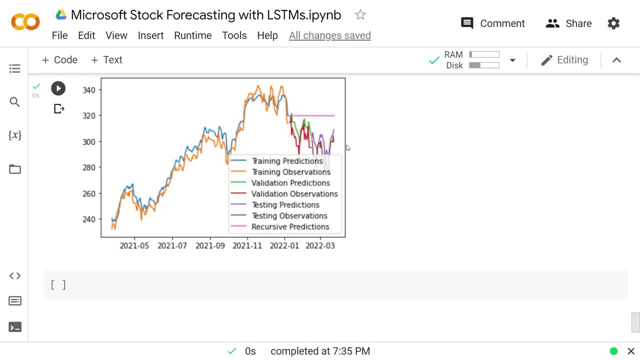 but on a micro scale. it's important to know as well. So I hope you enjoyed that video. if it brought you value, please drop a like and consider subscribing. it really, really helps and I'll see you next time guys.